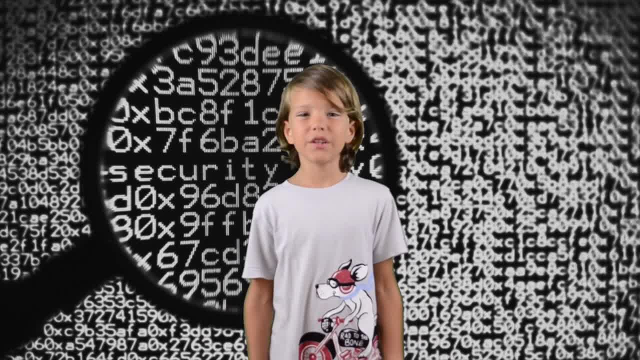 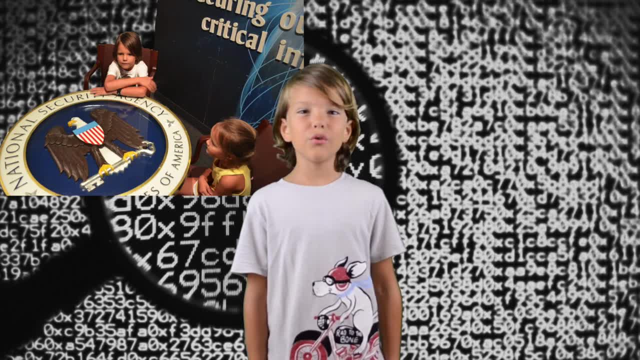 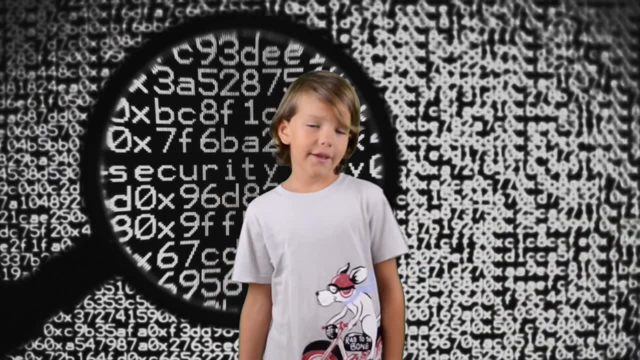 excited by playing around with this machine. so I decided for a deep dive about even more about cryptography. So I even went to the National US Cryptography Museum, which is standing right next to the US secret agency, And you're going to see it in today's video also. So 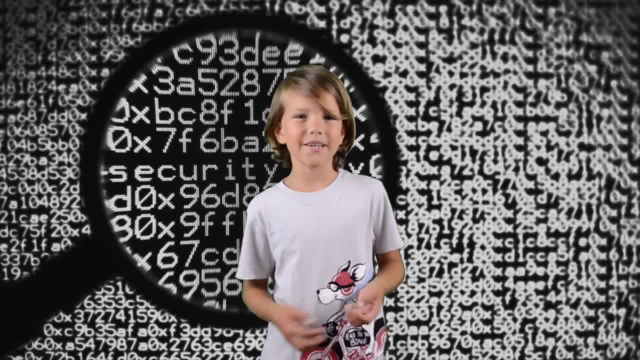 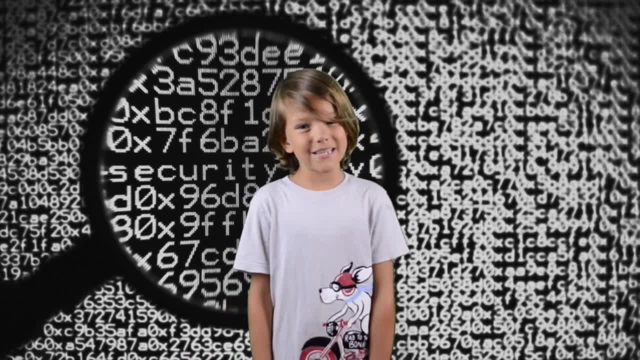 today. I'm going to tell you what cryptography is and why it is important in engineering and computer programming. I'll show you how to do it. I'm going to show you how to encrypt your message and send it open, but nobody will know what it says. 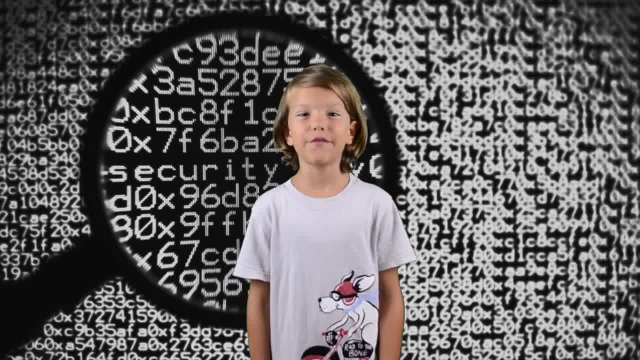 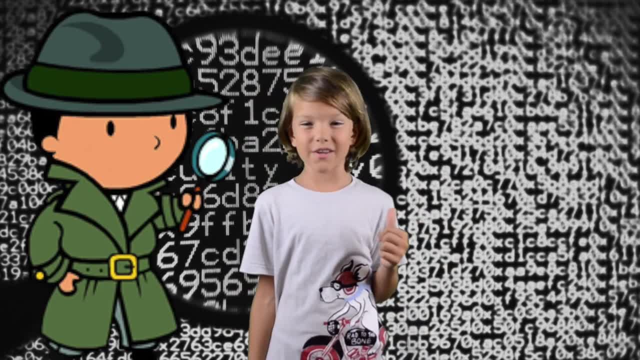 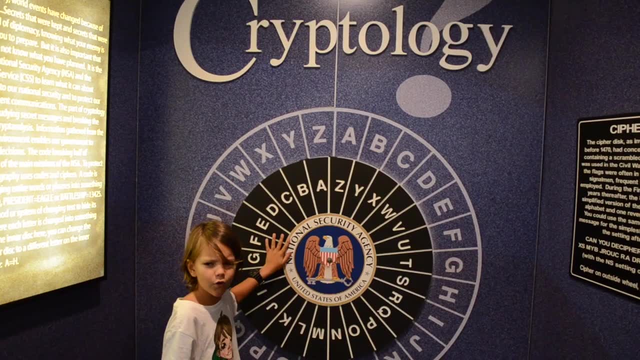 I'm even going to show you how to make your own cryptography machine. Isn't that cool And ta-da. If you watch my video very carefully, I'll tell you the instructions later. you have a chance to win a $25 Amazon gift card. 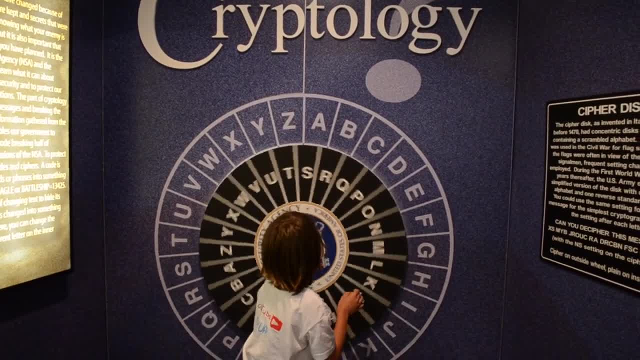 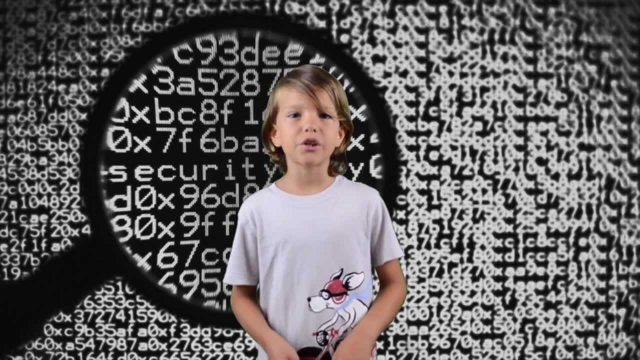 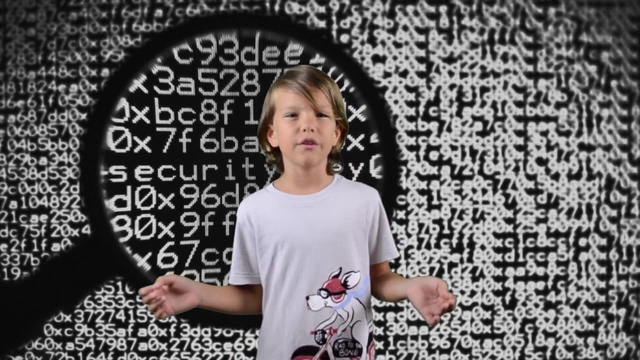 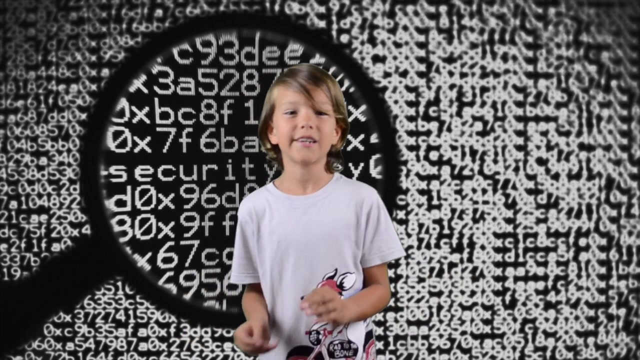 So what is cryptography? Cryptography is a technique for secure communication when everyone else can see it, Which means, even though people can see what message you are sending to somebody, they�re not going to know what message is written on it, because you may have your own letters. 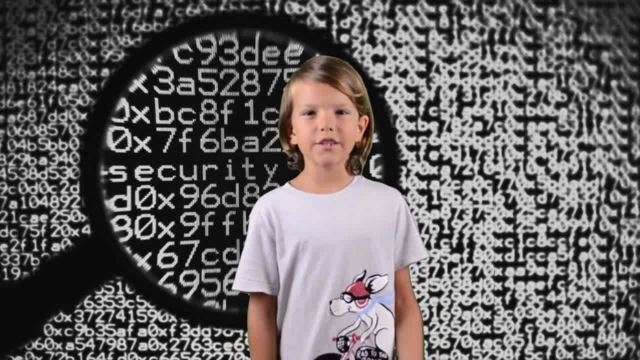 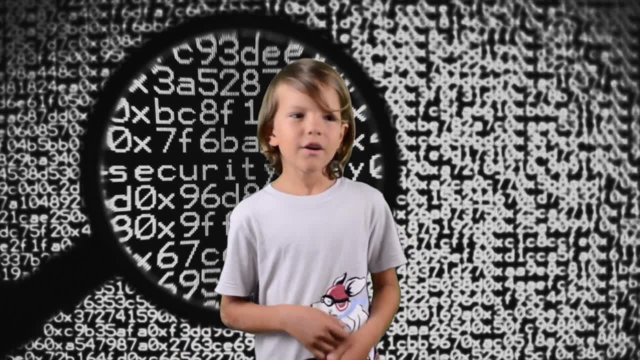 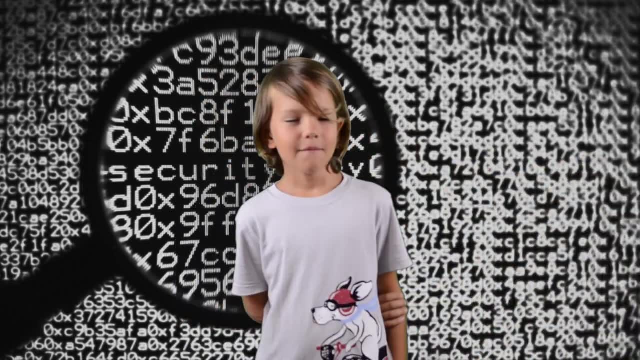 For example, I want to tell my sister what the message inside the candies is, but I don�t want anyone else to know where they are. first thing i can do is just tell her is just whisper it on her ear. but that's not going to be cryptology. but what if i can't whisper it on her ear? what if i have to? 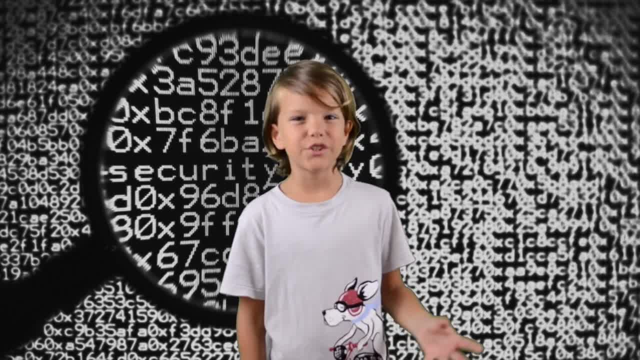 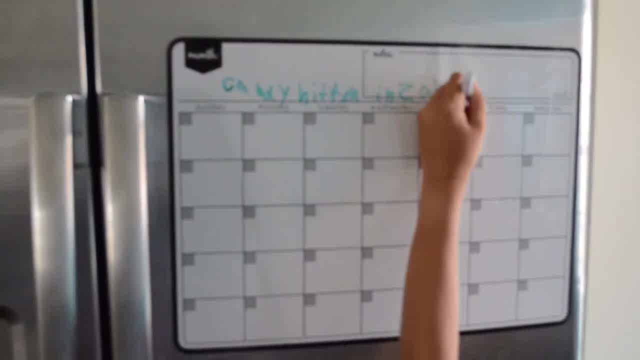 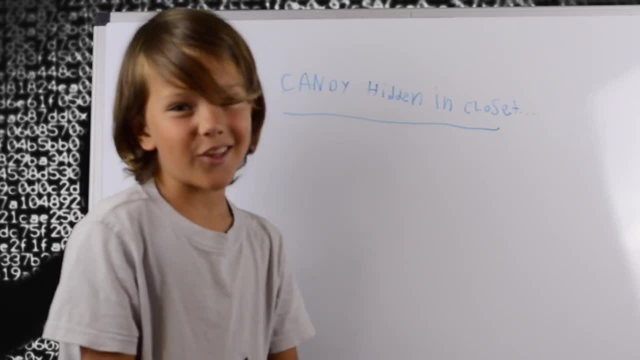 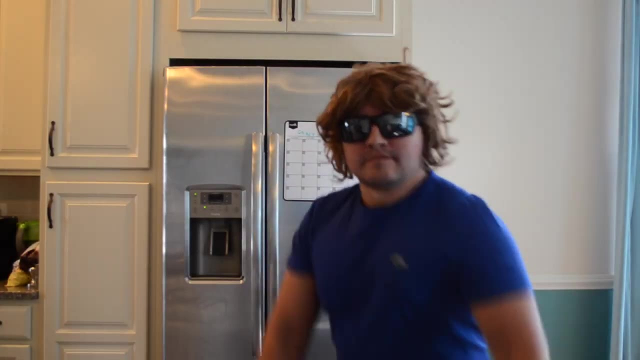 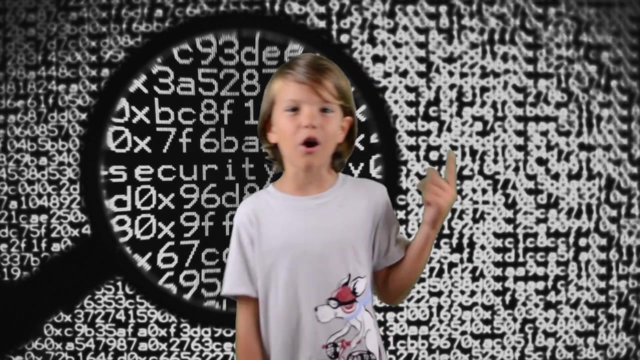 write it to her, for example, a message on our refrigerator, but i don't want my dad to know, to see this message, because he loves candy and i don't want him to eat all of it instead of my sister, and this is where cryptography helps us actually. 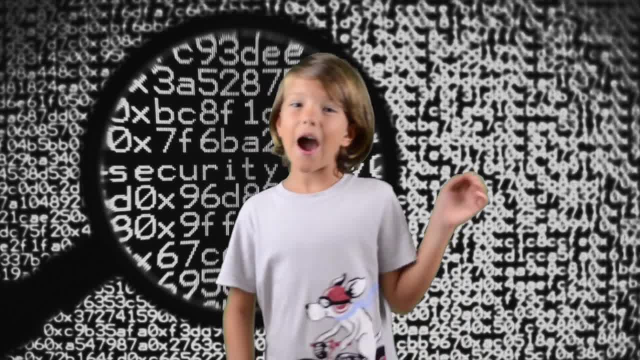 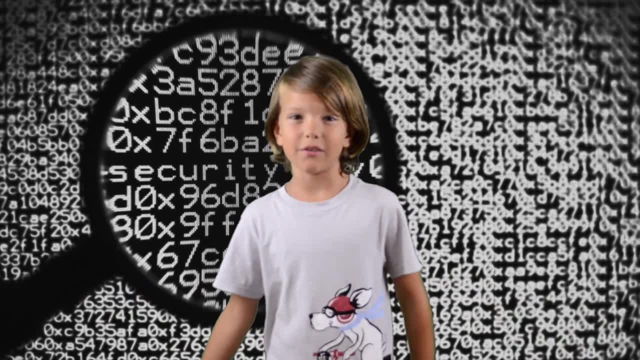 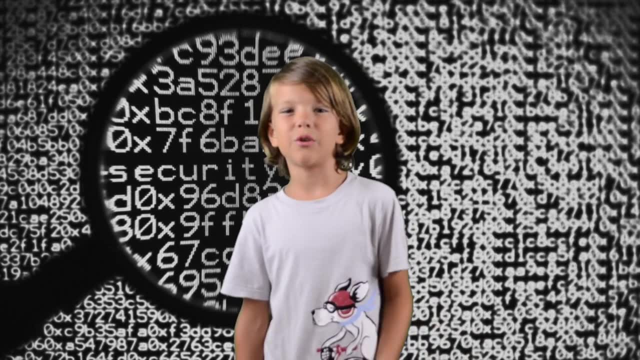 people have been trying to solve this for thousands of years, and- and of course i'm- and cryptography has a really long story, but of course i'm not going to tell you all the whole story, but you, but you can, um, but of course you can always go search up on google if you're interested in cryptography. 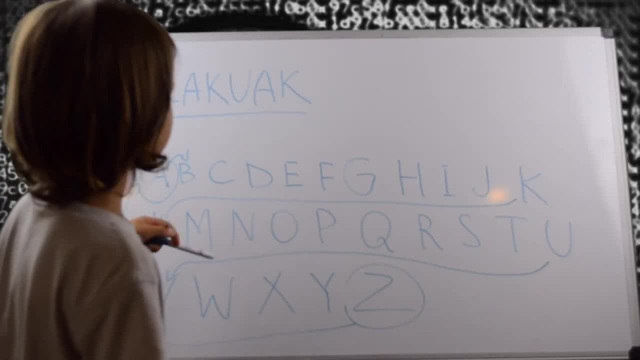 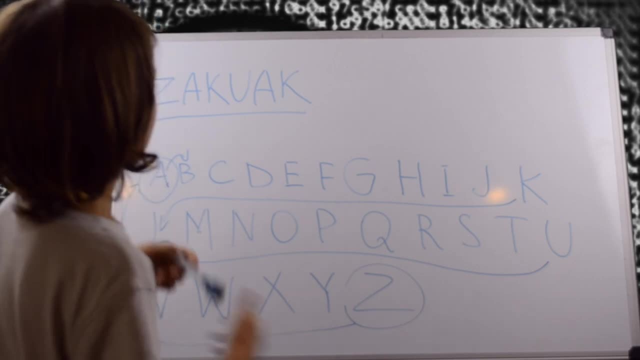 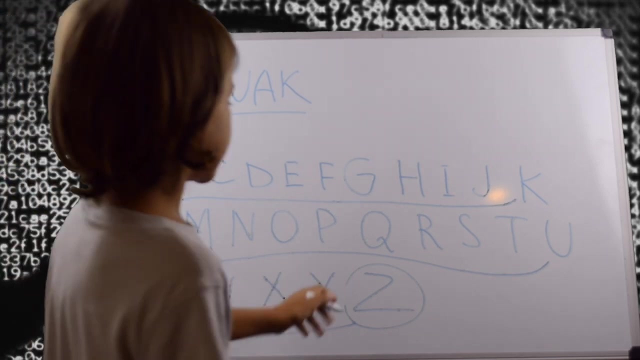 like me. so the easiest way to encrypt your message is to just change the letter to the next one in the alphabet. for example, i want to. i want to encrypt my. my youtube name is zach uac, so uh, first i take a look at z. z doesn't have an. 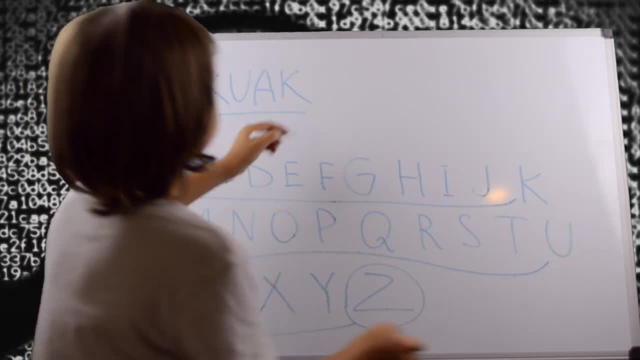 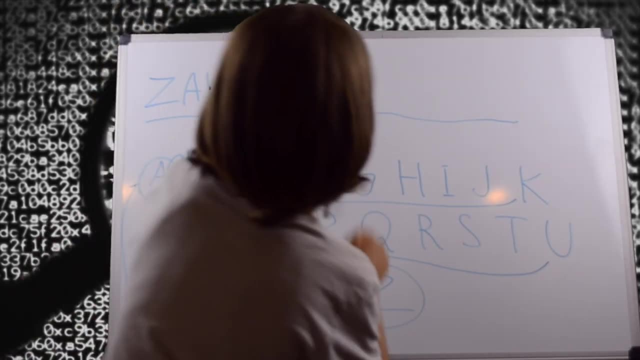 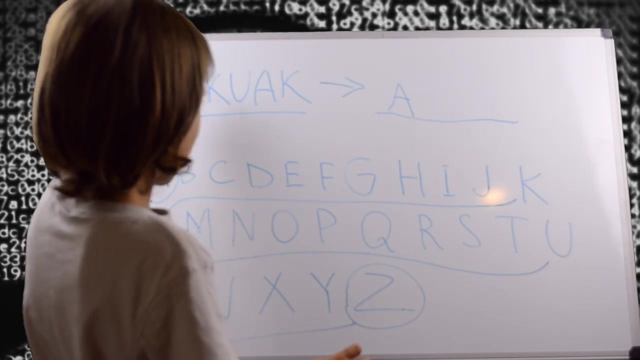 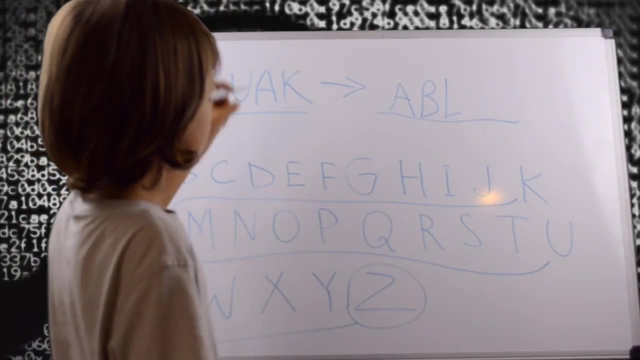 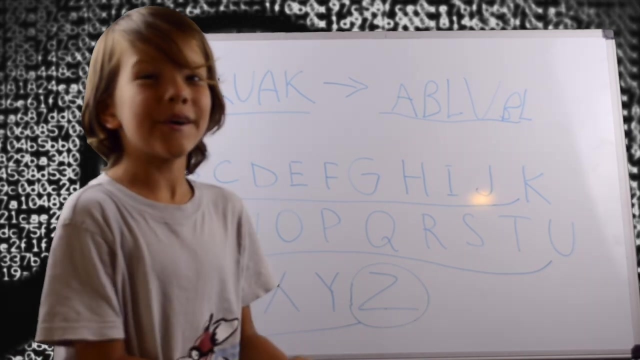 x letter, so we change it to a. so here's the encrypted version. oh sorry. and then the a from zach turns into b, a b. next is the k, so the k turns into the l- avovable. isn't that a funny name, well? well, when you encrypt your, when you encrypt messages, it. 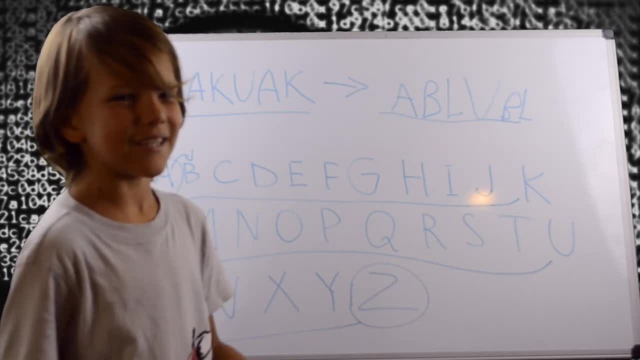 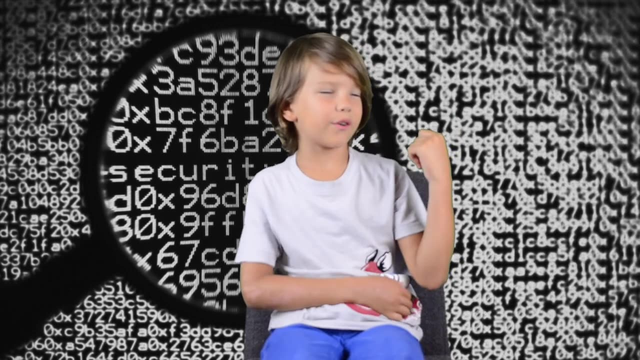 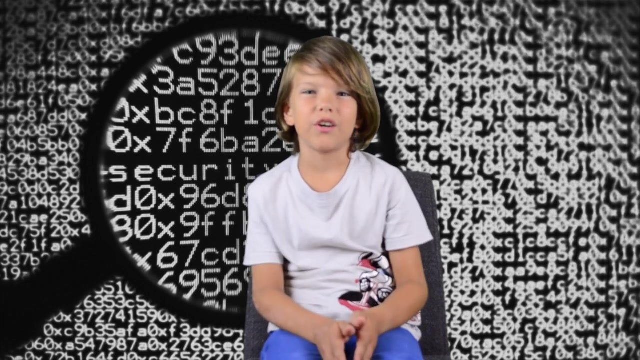 usually turns into a pretty fun, into a message. that's pretty funny. but sure, the technique is pretty simple for uh, encrypt for uh. when we encrypted my, my youtube name, right, so, uh, it would be pretty easy for someone to decrypt it. but what if now, instead of changing the letter to the 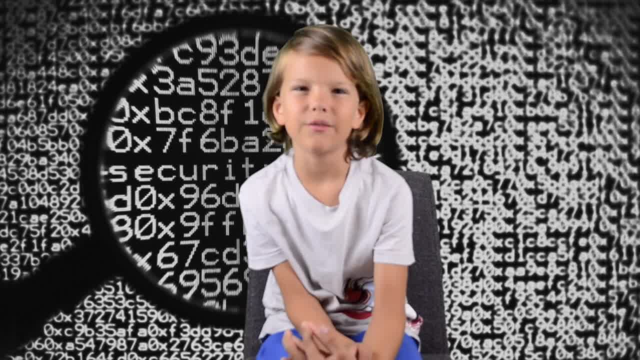 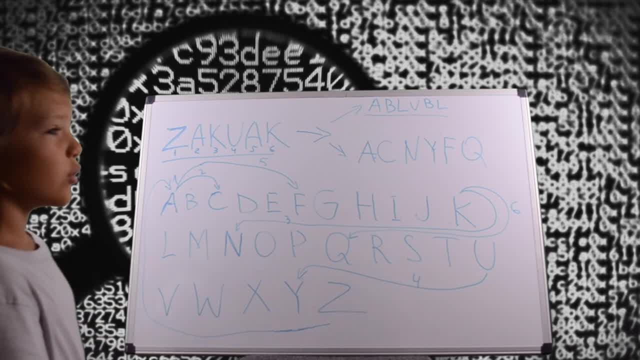 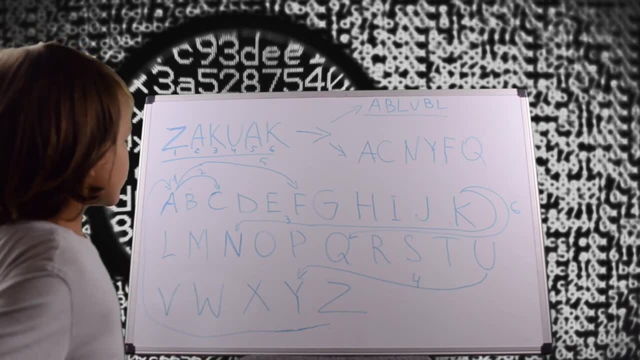 next letter of the alphabet. just make something out, make up something else, so here will be a harder way to encrypt, to encrypt your names, so, so it's going to be harder to encrypted. so, for example, we can use, we can use a technique: uh, every, let the position of the letter. 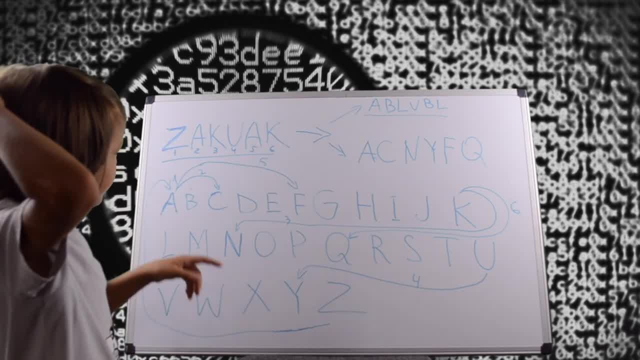 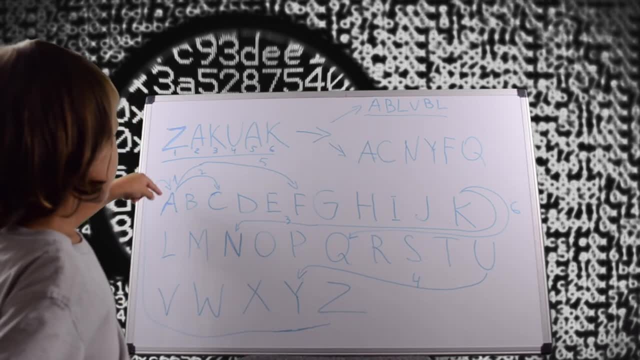 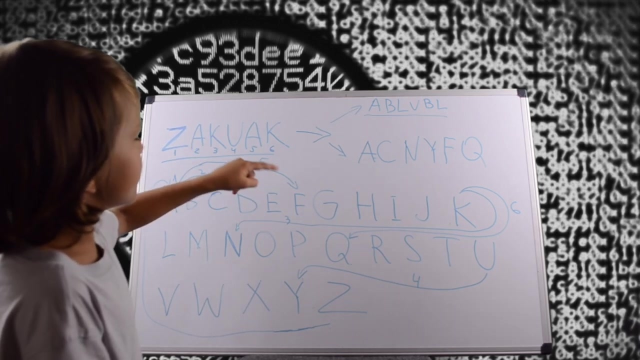 in of the letter in the message and in the alphabet. for example, the z will be the next. the next letter from z is a, so first letter will be a next, next letter is a. its position in my name is number two, so we go to a one two. so that's gonna. so the a is gonna be be turned into a c. 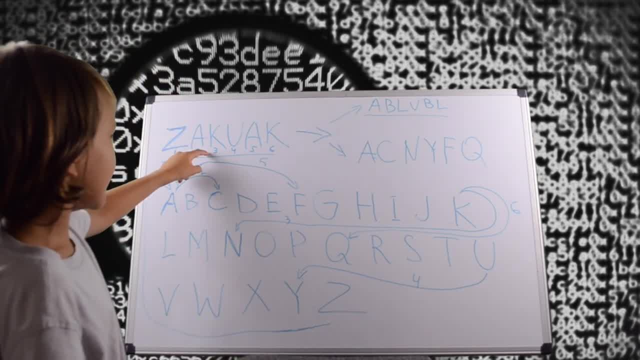 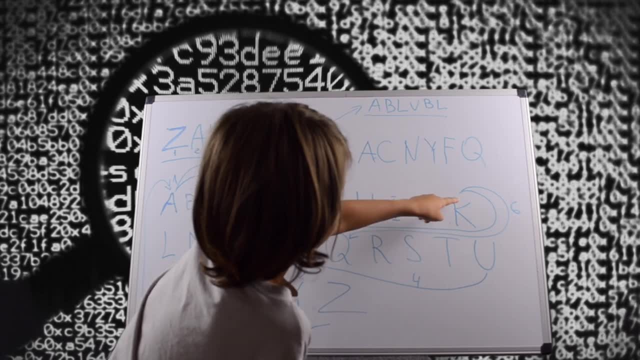 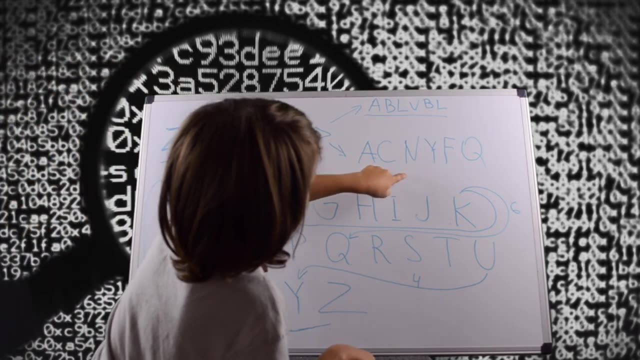 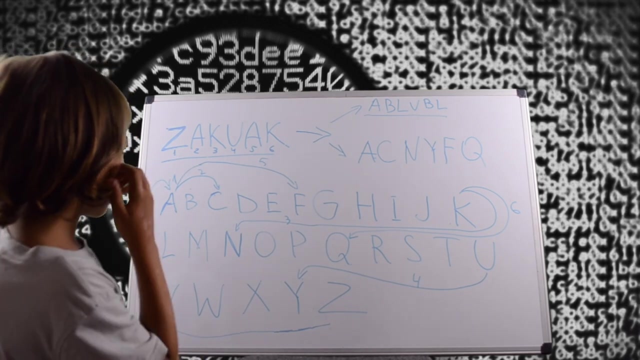 then next letter. next letter k, which is third position. we go to k, so k is in third position. so we count on one, two, three, so the k turns into a n. next up is u. u is fourth position in my name, in my youtube name, so we go to u. 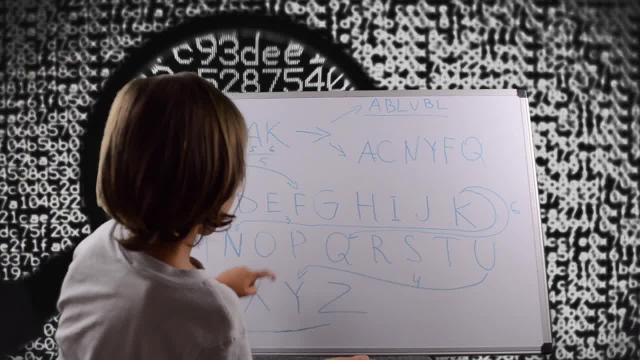 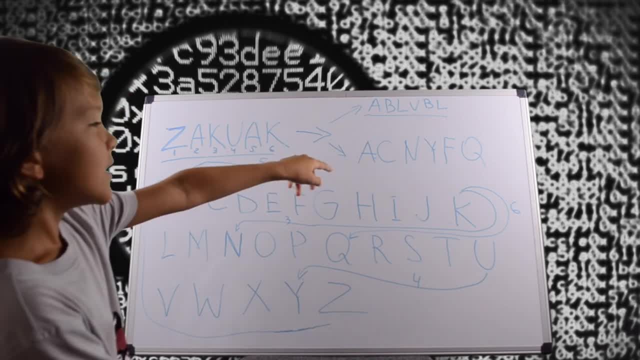 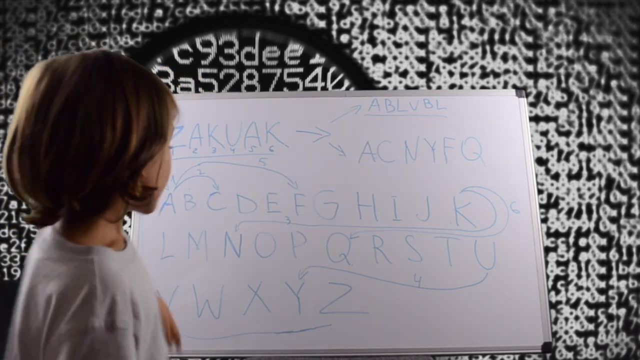 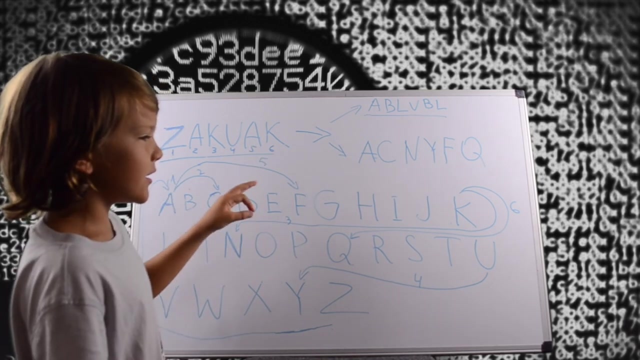 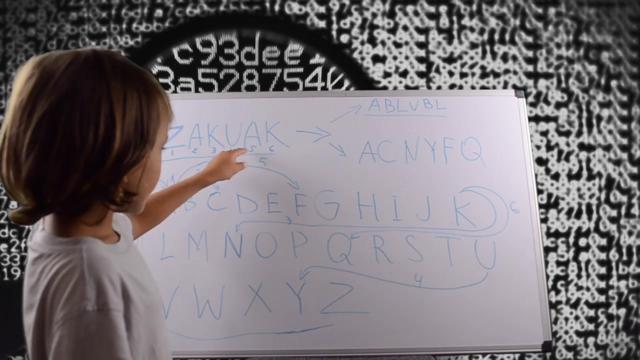 one, two, three, four. that turns into a y. then next is a and this, and see here the a, the, the repeating, the repeating letters are exactly the same, but here they won't be the same because they have different positions in the name, which means a different let different letters, that they get encrypted in, and I get encrypted so. so the next a is fifth. 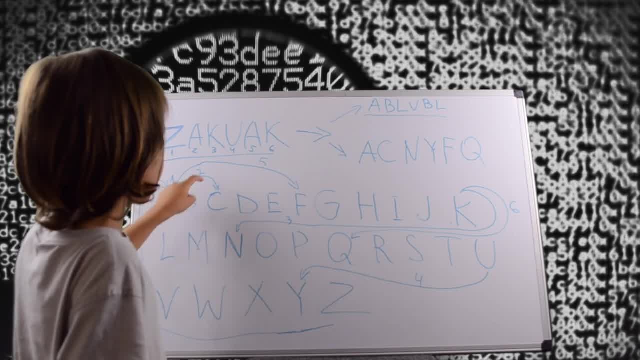 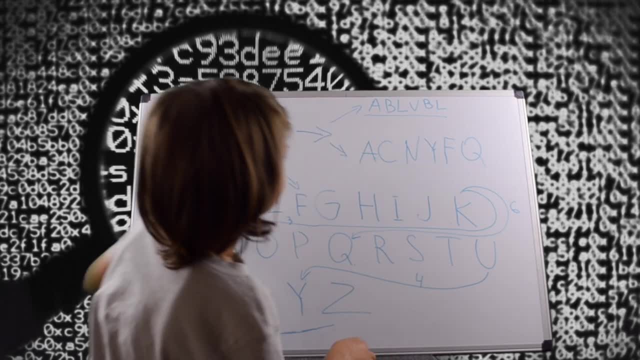 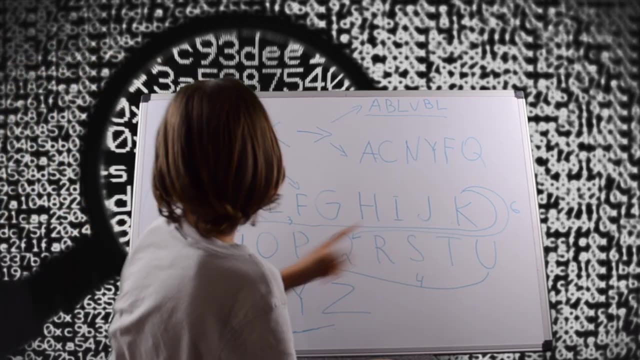 position, not second. so we go to a one, two, three, four, five, which turns into an ad instead of a, a, C, and then the last letter is the sixth K, so we go to K 1, 2, 3, 4, 5, 6, Q, so 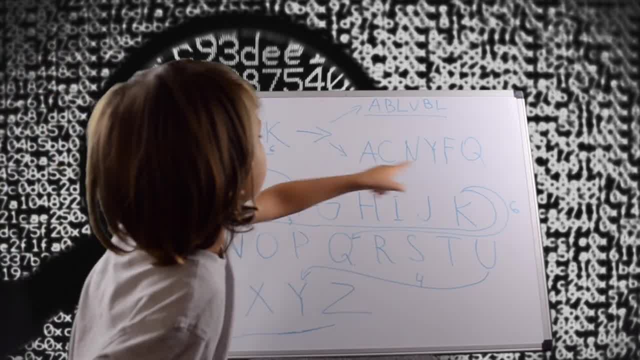 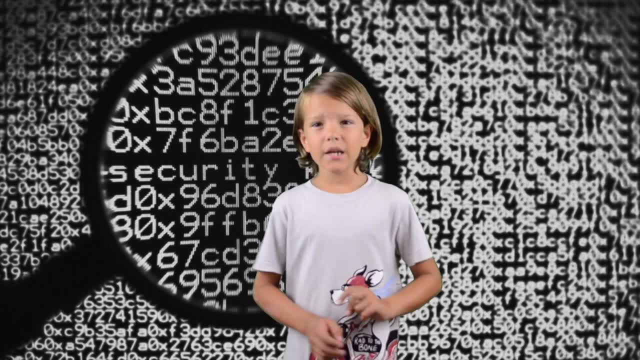 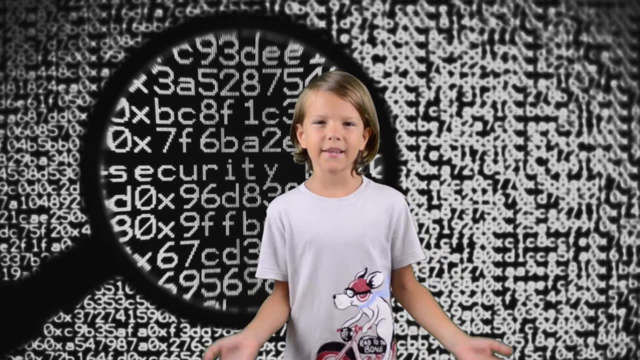 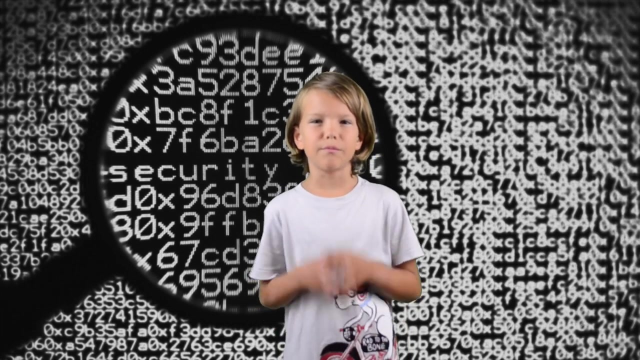 this is my, so this is my whole encrypted name- in the harder way. of course this second encrypt was harder than the first one, but a person, or especially a computer that can do that- can run millions of operations in a second- can easily decrypt it. but before I tell you one of the best and most modern, 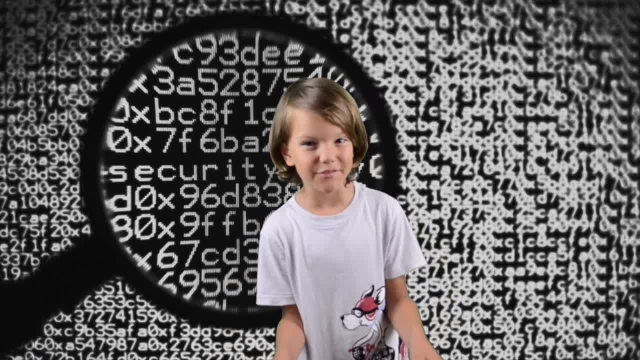 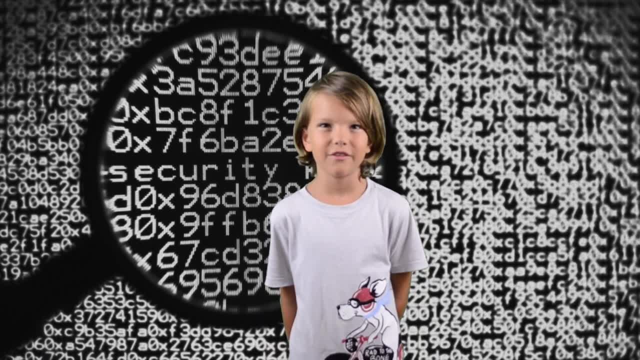 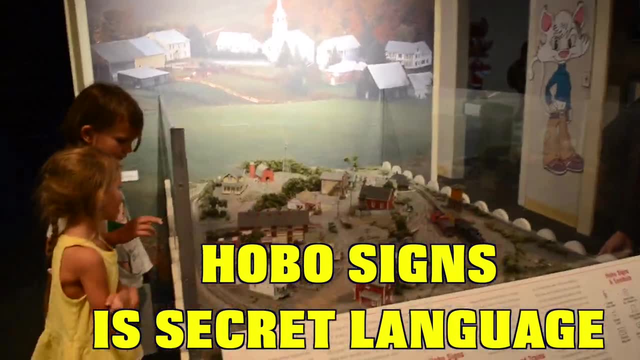 techniques of cryptography and how you can earn lots of money by just finding a certain number. let's look into the National Museum of cryptography cryptography. this video will be from the National Security Headquarters, so let's talk about cryptology. so what are hobos? they're basically just. they're basically just signs that. 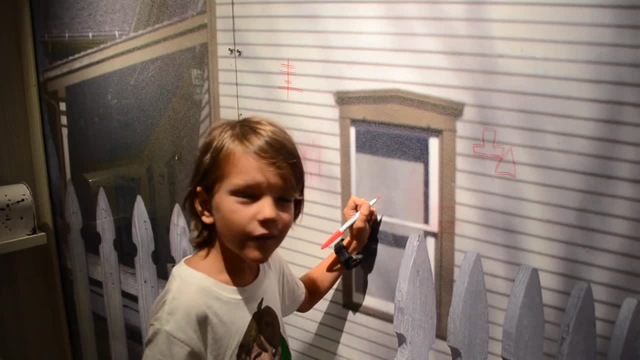 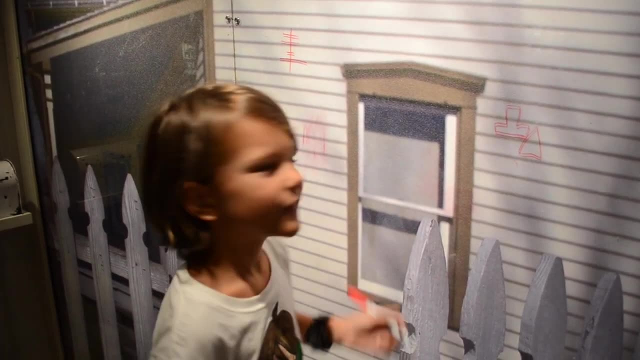 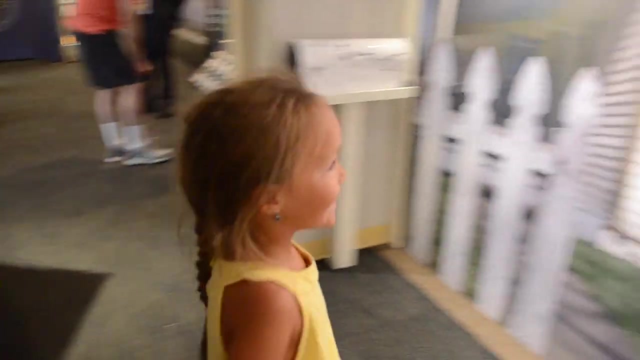 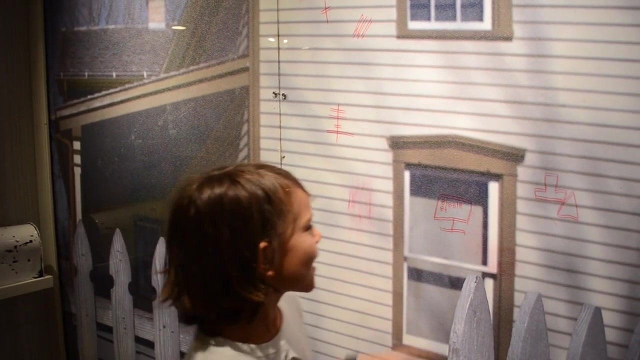 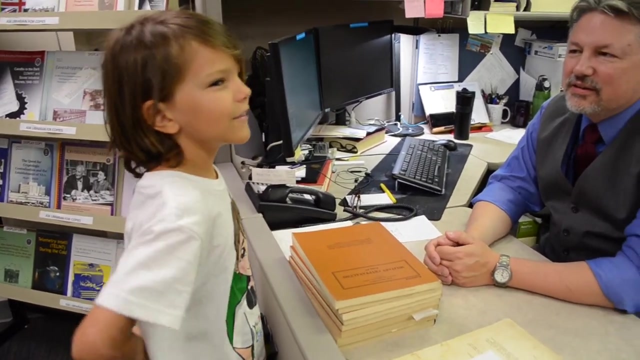 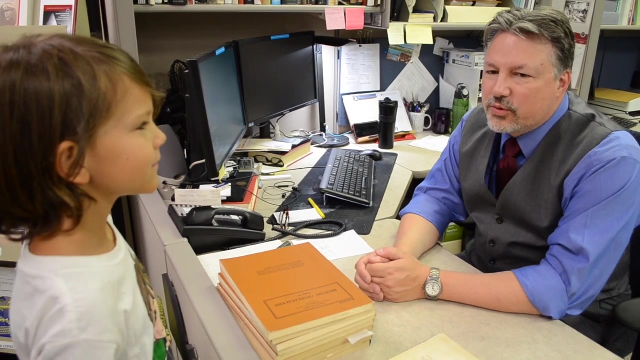 people made up to talk with each other. right now I'll make up a sign that means that says that means the programmers live here. this is how this is a library. yes, are these all books about cryptology? they're mostly books about cryptology. there are a few books in here that we keep for context. 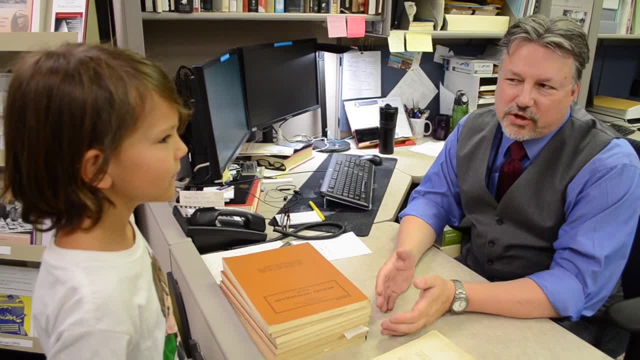 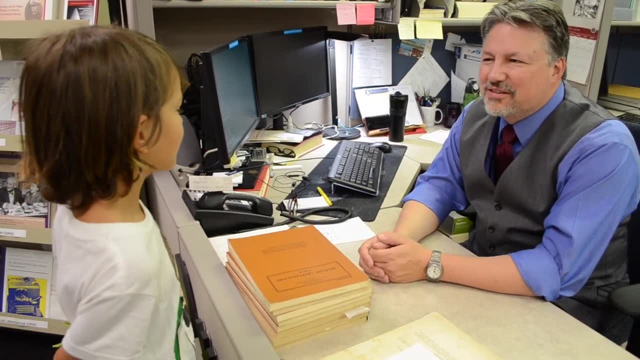 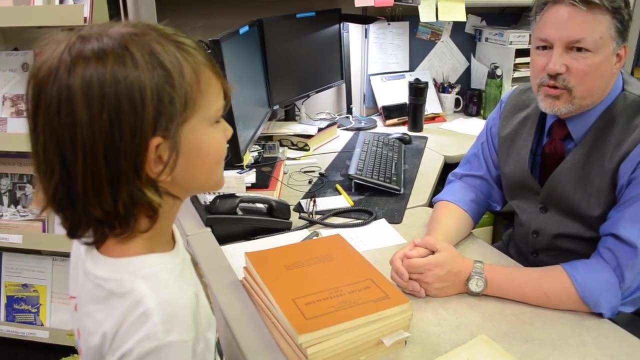 so if someone's in here studying cryptology and they're also working on World War two, we have books about just general books about World War two also, or World War one or other things, you're welcome. do you know how much books this library has? we have quite a few. we have over. 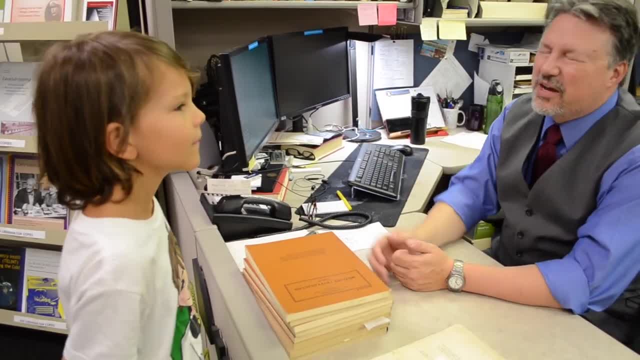 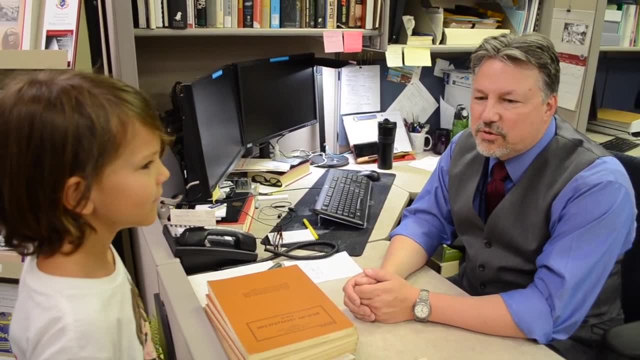 10,000. Wow, some are in here and some are in the back. what book would you recommend for a kid to read, like about cryptology? oh, there's, there's a couple. so there's some fiction books that are really good. there's a series- my daughter- 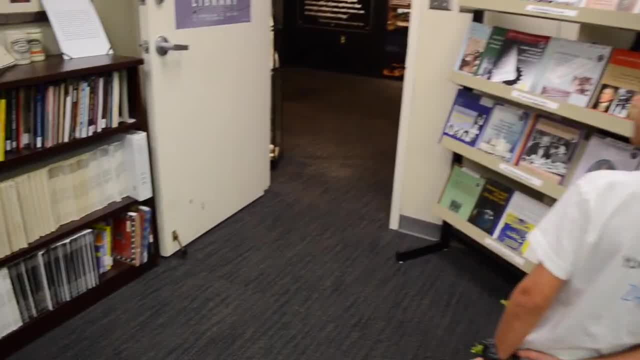 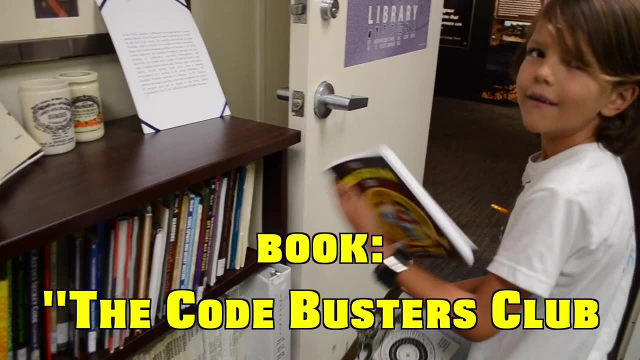 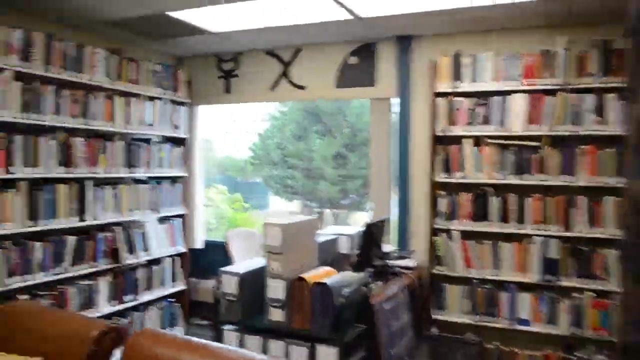 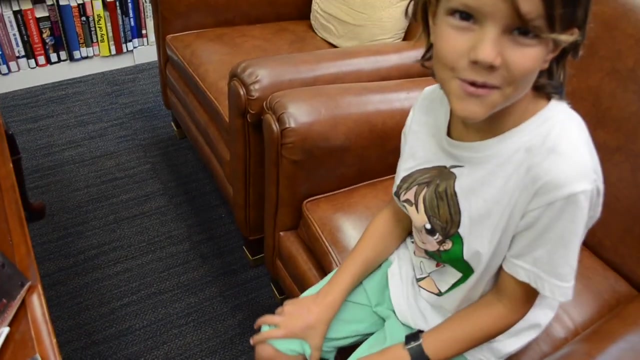 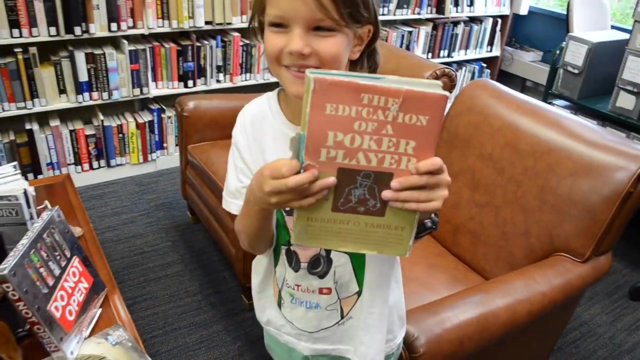 just read. if you look at the last three books on that top shelf: oh, this is definitely a book about crypto, cryptology. it says: do not open, but I'll try. they even have a book for my sister. she loves playing card games and this is an old computer. 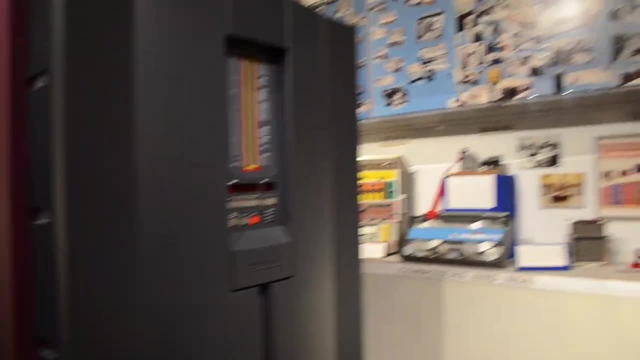 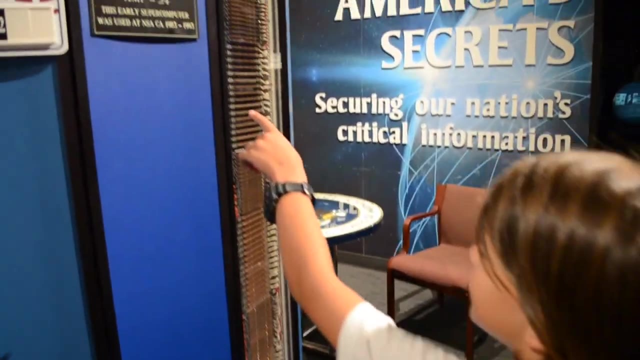 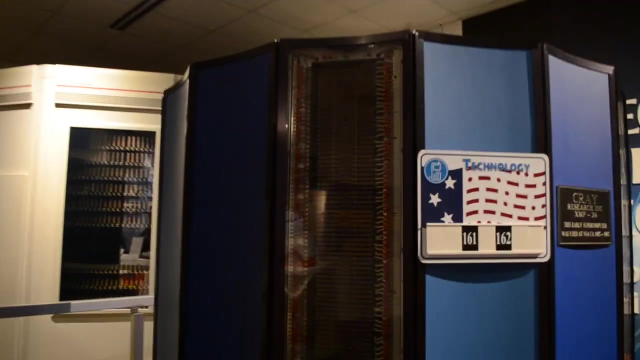 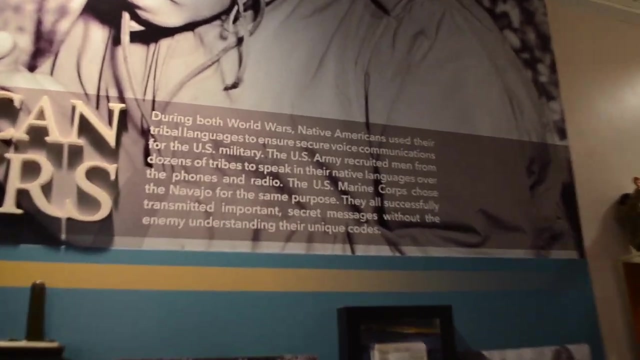 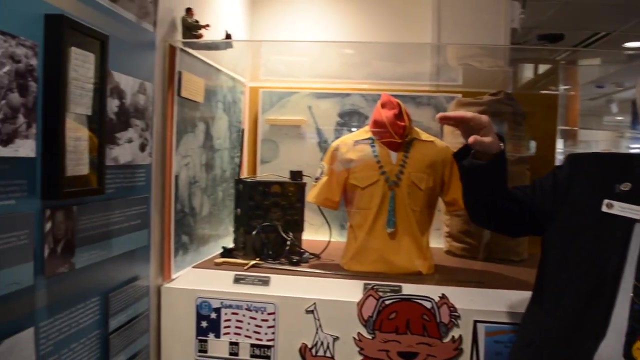 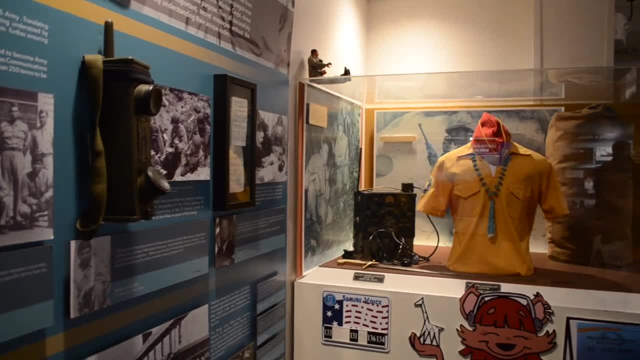 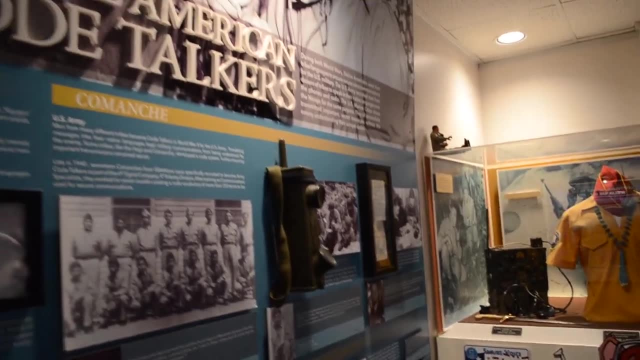 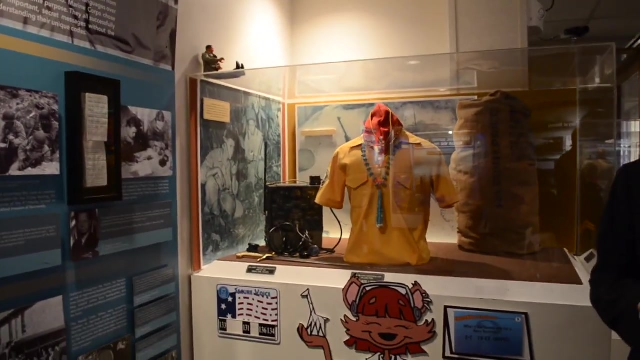 went to- I think it was in the 19th century, World War II- and the most famous one is the Navajos, and so the Navajos had. one of the things that was unique about the Navajos is that Navajos had no written. 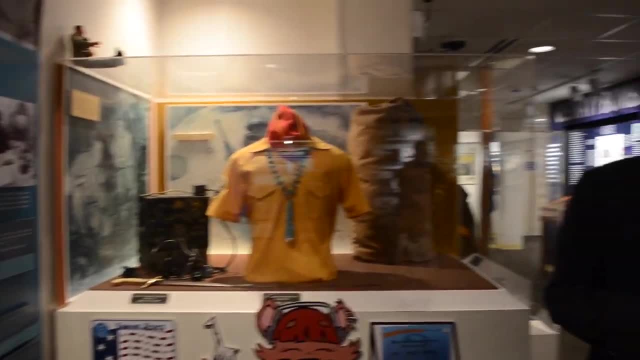 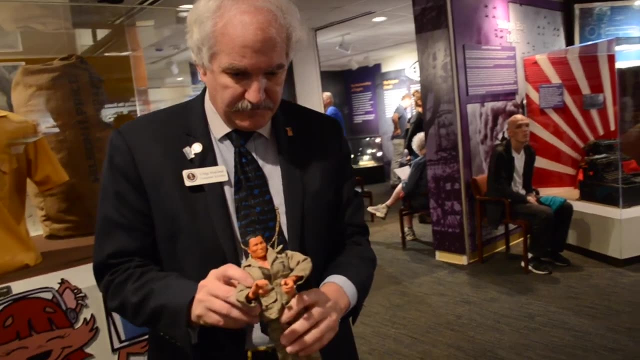 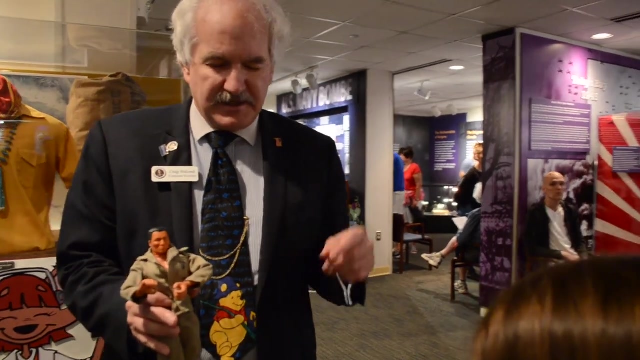 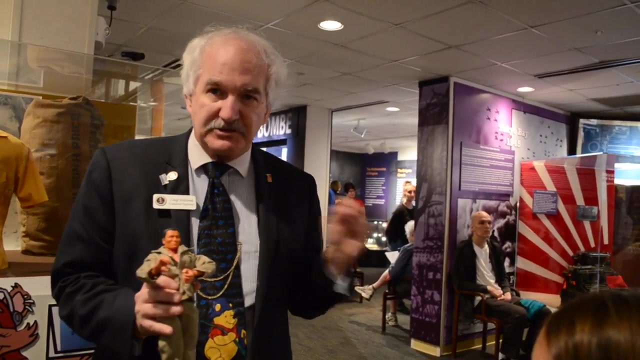 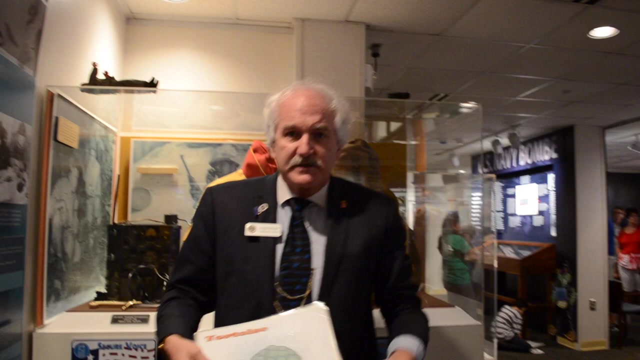 no written dictionaries. they had never written anything down. this is Navajo Joe, so this is what they would actually say, but there are a lot of things that they, as they were trying to figure out what to talk about. they didn't have a place in their reservation that talked about various things like that, so so I have to. 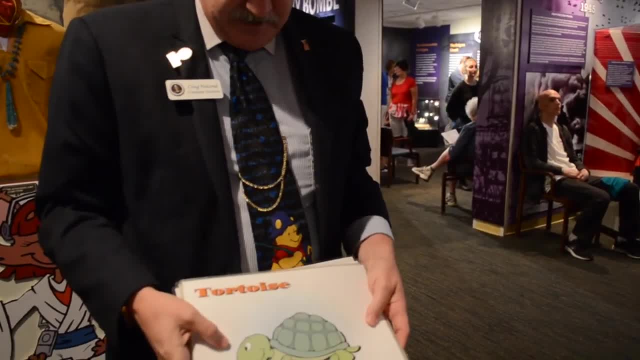 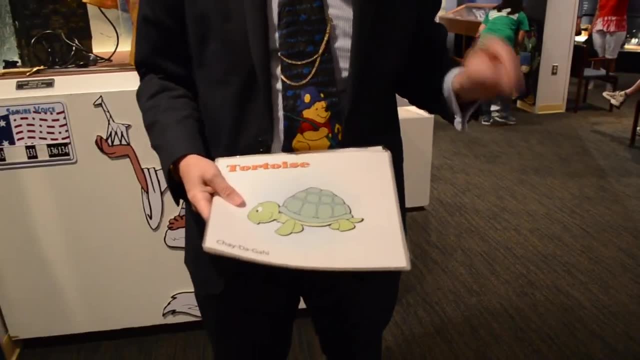 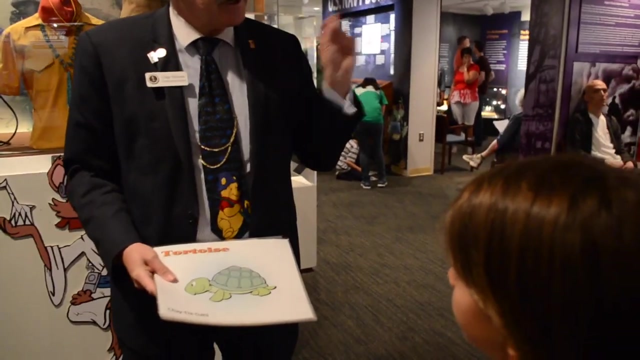 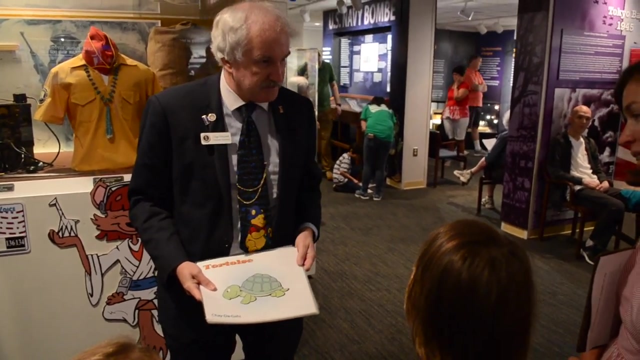 come up with other things, like they would say something like tortoise. what do you think of tortoise represented okay, so what do you think it would represent in the military? it's green, hard, slow. so there were no words tank in the reservation. so they said: request tortoise support. how about iron fish? 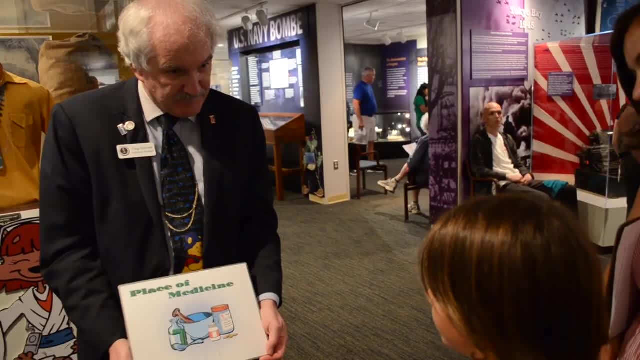 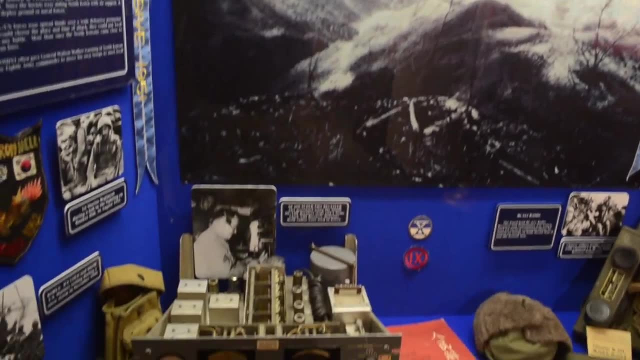 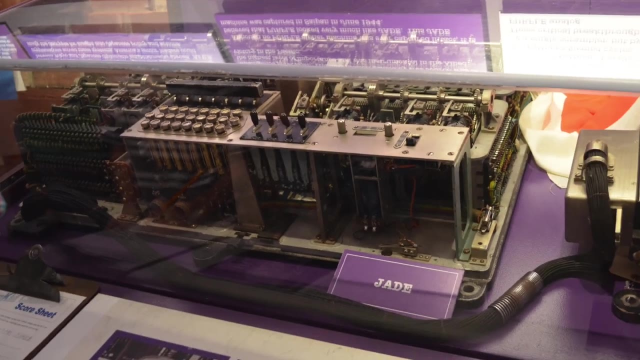 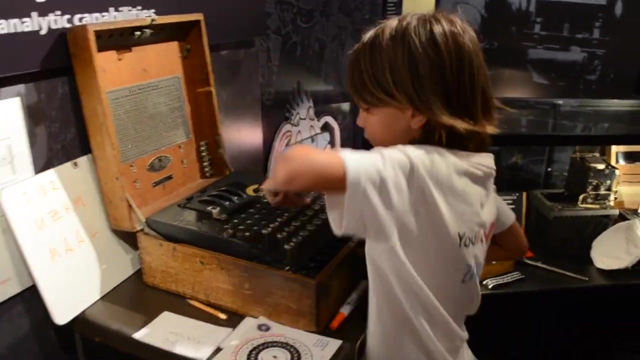 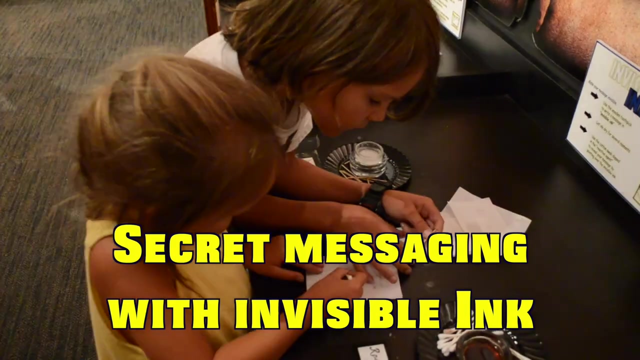 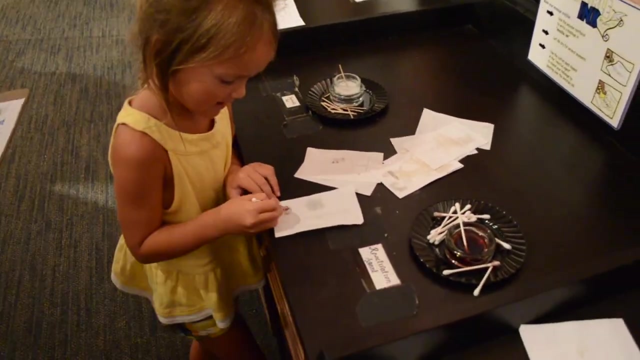 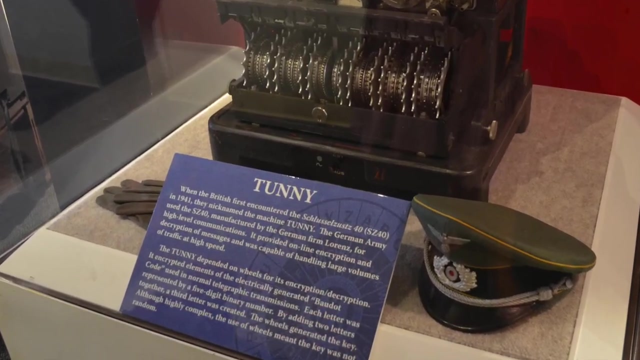 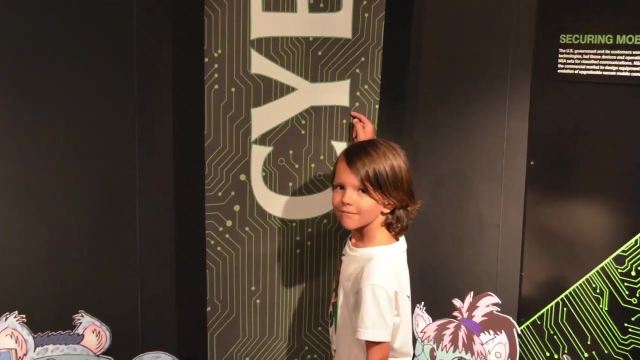 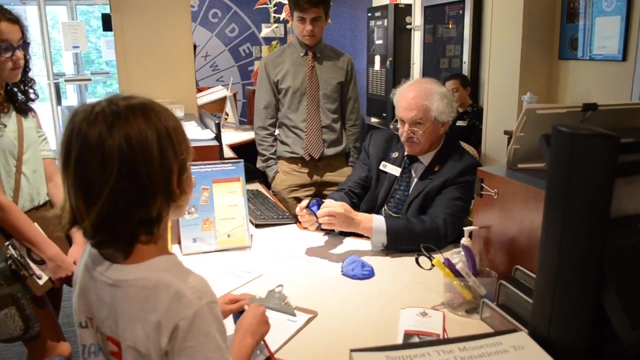 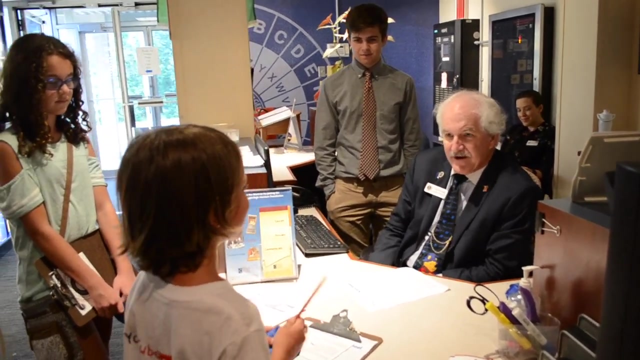 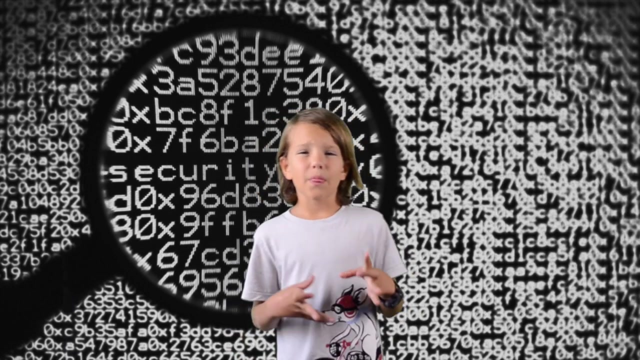 submarine, very good hospital, very good general. so, yes, so so, and now very, the town, the town, the town. that yeah, town, town, town, town, town, town. This was one of the best museums I've seen here. Alright, well, I'm glad to hear that. So, as you can see, all the techniques we saw always need a key. 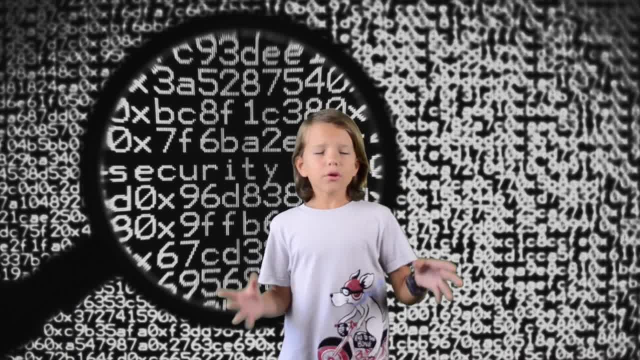 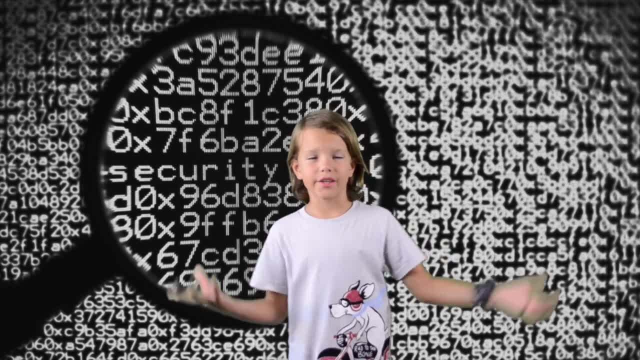 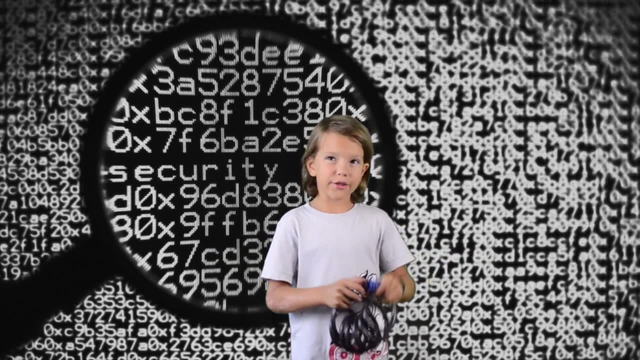 So for secret communication- both people that are talking to each other- they both need a key. The key is called a secret key. So same with a locker, for example for your bike. I need to give her the key to open it right. 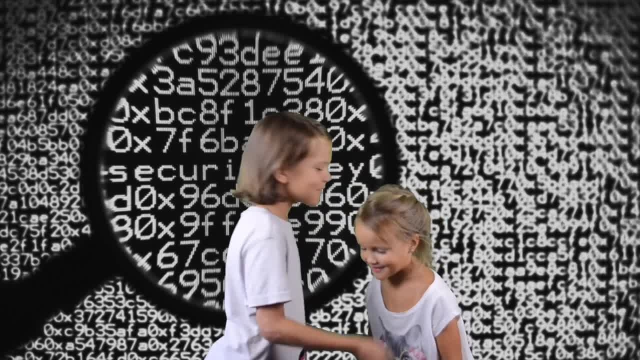 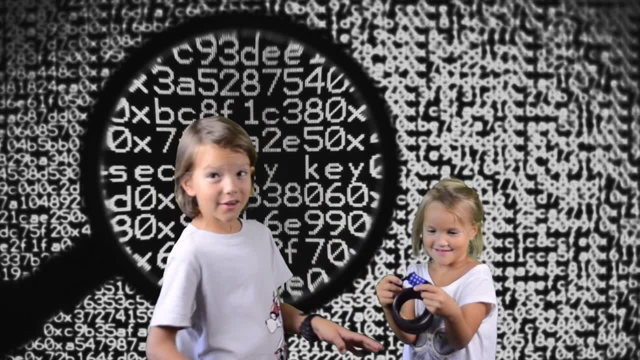 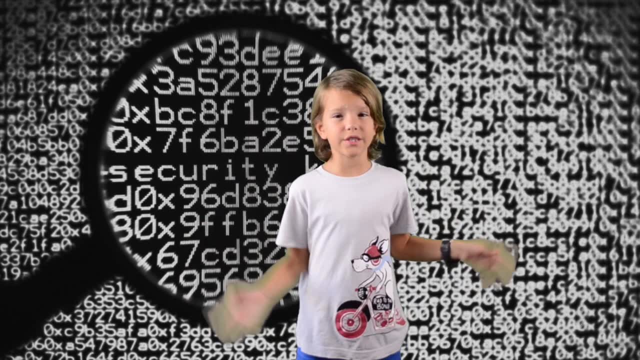 You see, only she can unlock it, but no one else can unless I tell them the code. But what if I can't see my sister every day to tell her the secret key? In this case I would need to send a key somehow to her. 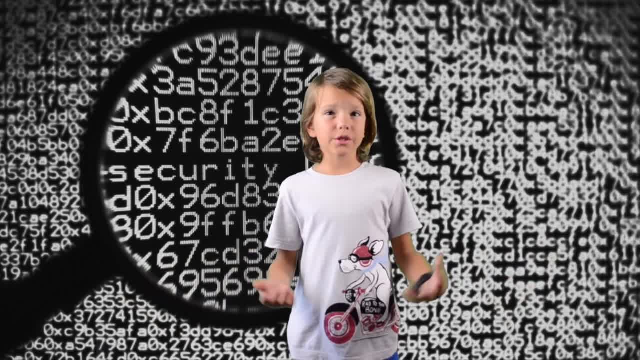 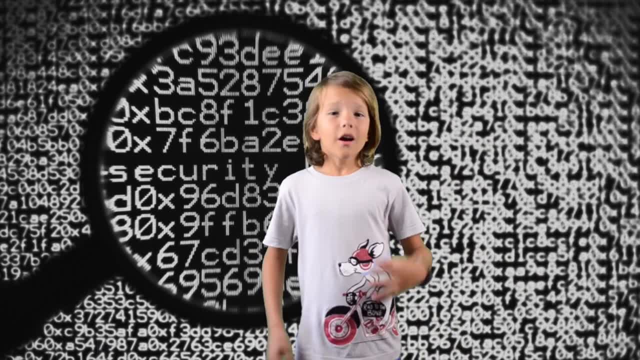 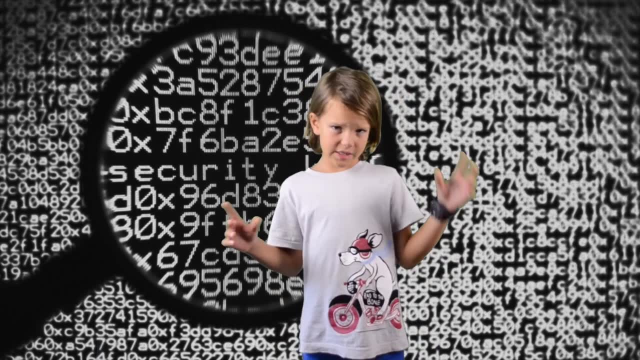 On the way. what if somebody gets it? Another person? he used the key with our communication To decrypt it. Here another technique comes to help us: Cryptography with two keys. This is actually a very complex technique. We use two keys. 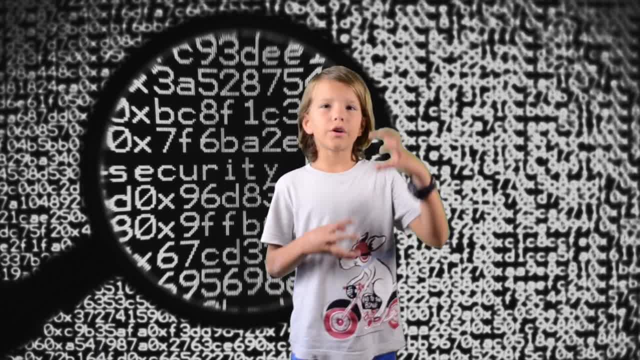 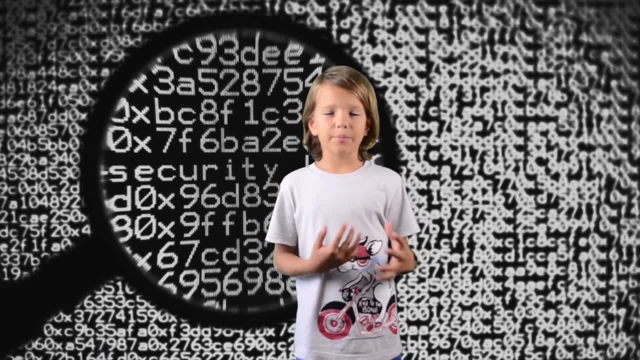 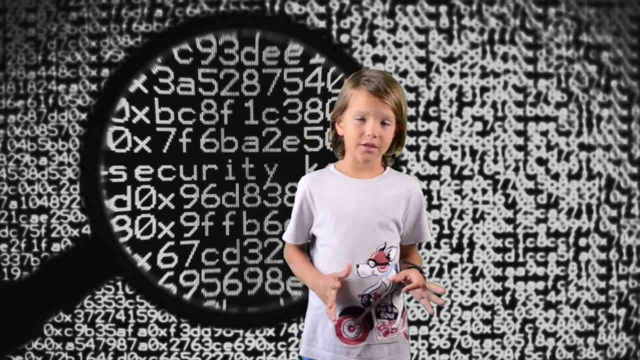 One is open and one is private, just for you. So the open key you can send it to anyone. So the message will be encrypted with the open key, But to decrypt it you can only use the private key. In this technique, prime numbers play a very important role. 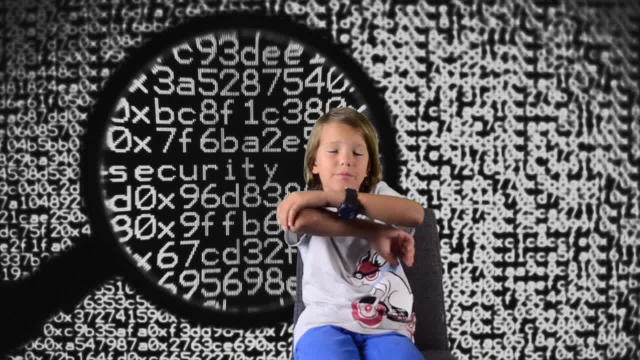 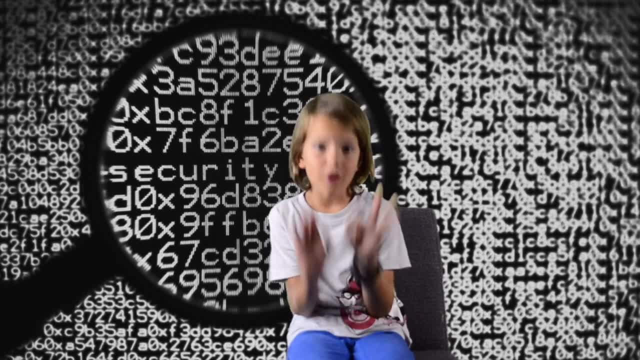 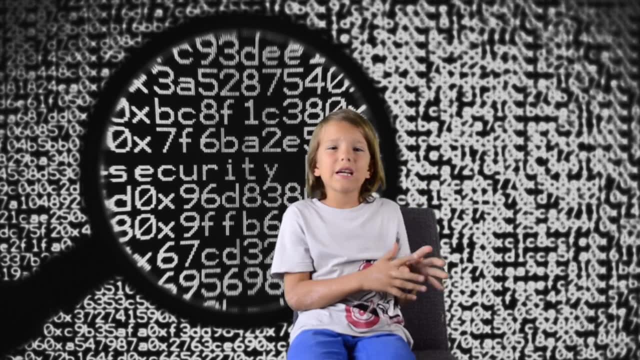 Believe it or not, this is what some people just do all the time: Search for the next prime number. And, by the way, you can earn a lot of money by By, By knowing, By, By knowing the next, The next existing but unknown prime number. 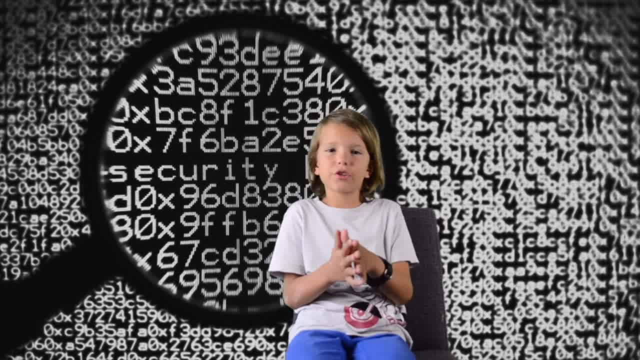 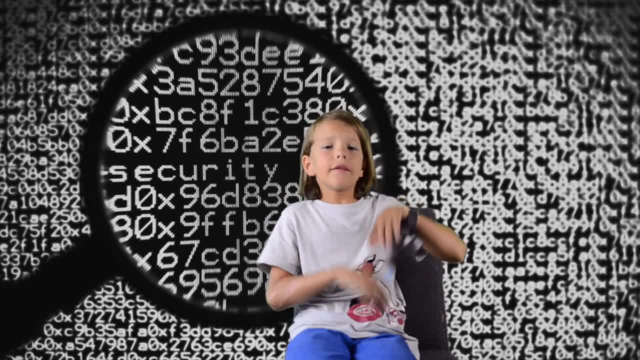 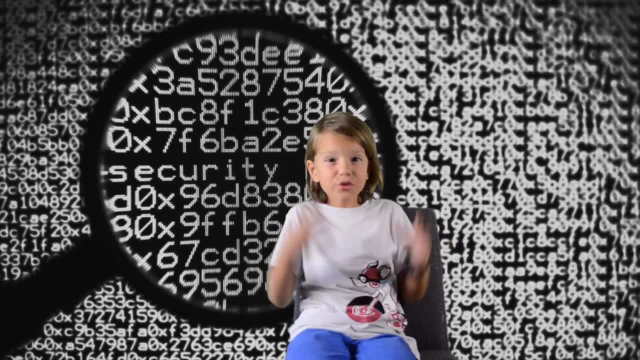 For example, in 2009, it was $100,000 reward For a prime number that contains more than 10 million digits, And the largest known prime number, as of July 2018, has more than 23 million digits. That's a huge number. 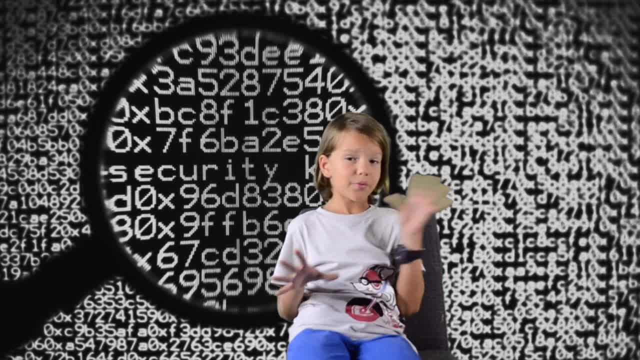 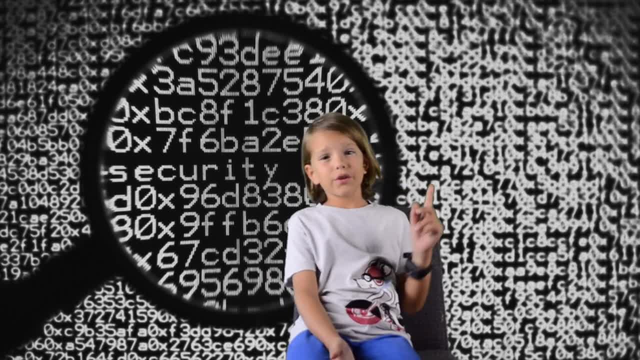 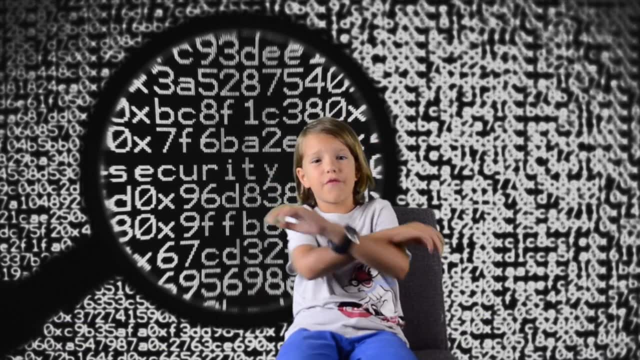 That's a huge number. So, as you can see, it is probably not an easy task, right? So if you are interested in this, you can just go on this website for way more information about it. Cryptology is also used very much in wars. 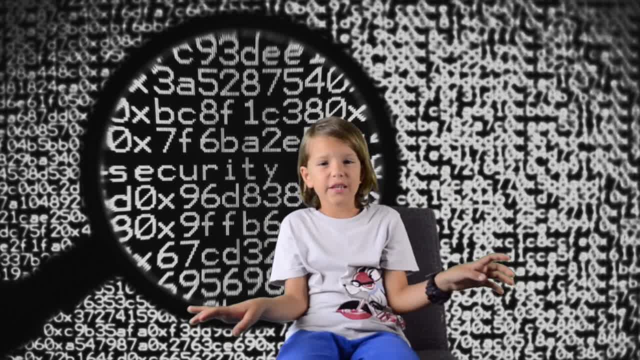 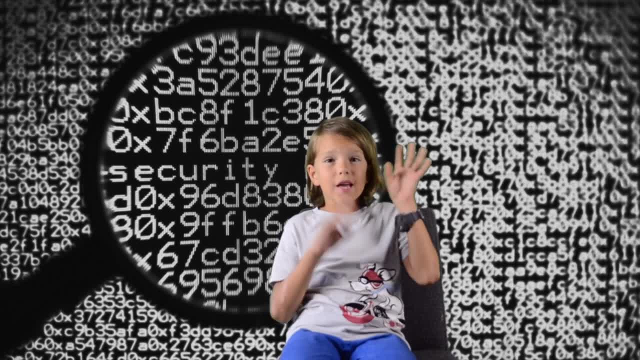 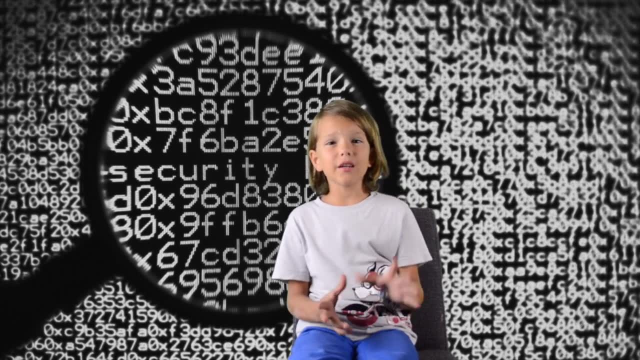 As you need to send a lot of things but enemies can't see it. I really recommend you to To read about the Enigma, One of the most important stories in cryptography. Enigma was actually. Enigma was actually the beginning of people making computers. 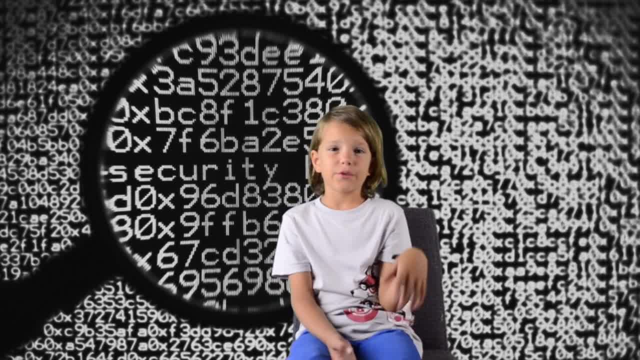 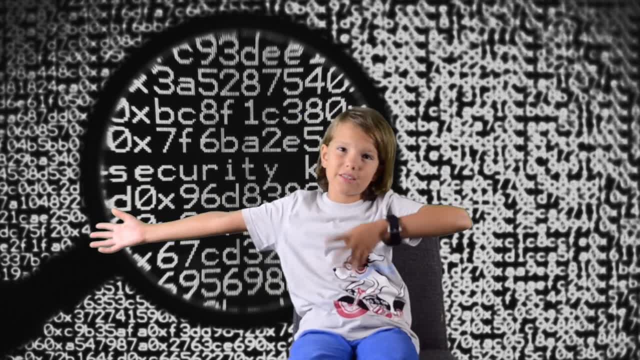 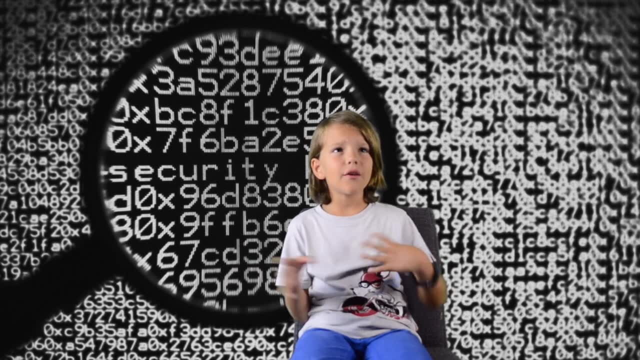 And, for example, a computer from now that we usually- For example that we usually use- is actually started its story way from the Enigma in the 1930s. Okay, Where is cryptography used for computer programming now? Right now, in computers there's a lot of private stuff being sent. 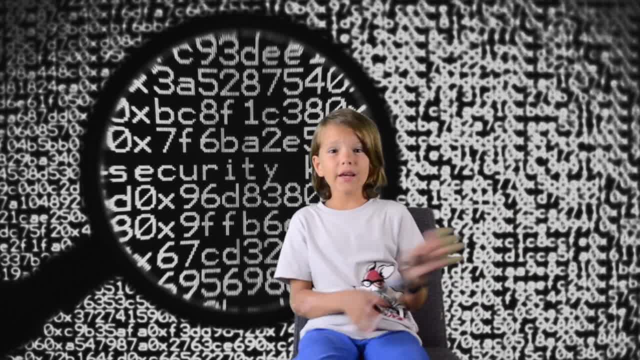 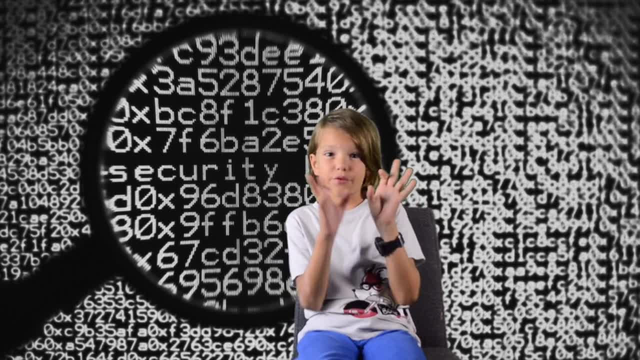 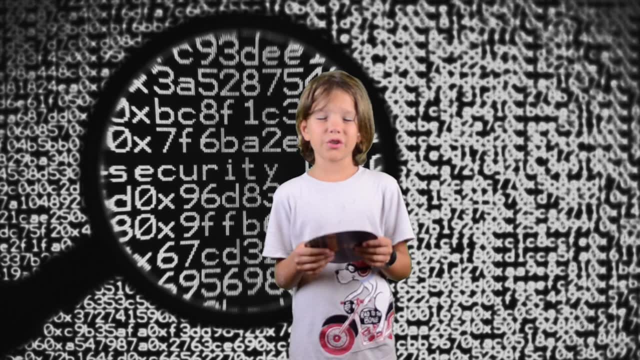 For example, money to banks, And bad guys can Might be able to hack it and And steal the money for crime. This is where cryptology helps. So, as I promised, I was gonna show you how to make your own cryptography machine. 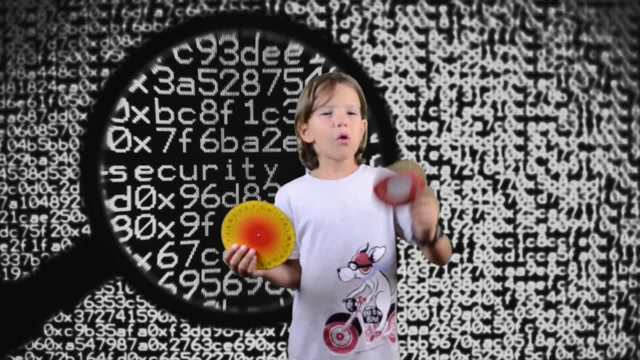 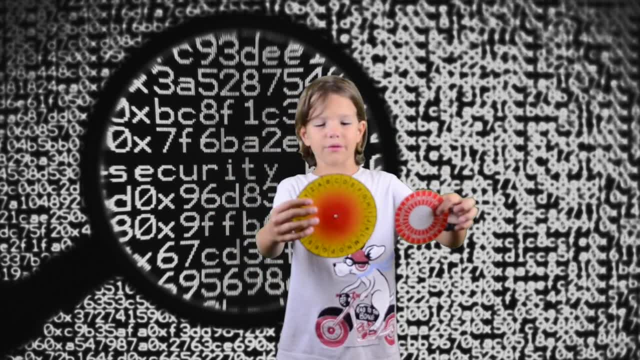 First you have to make, You have to cut out on a sheet of paper one circle that's a little smaller And one circle that's a little bigger. I've already done half of the work for you. If you just click down on this link below, you can. 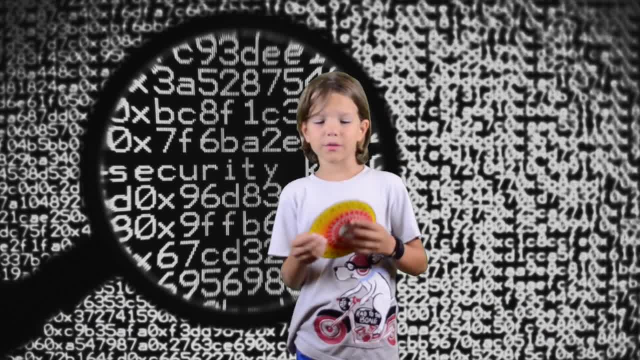 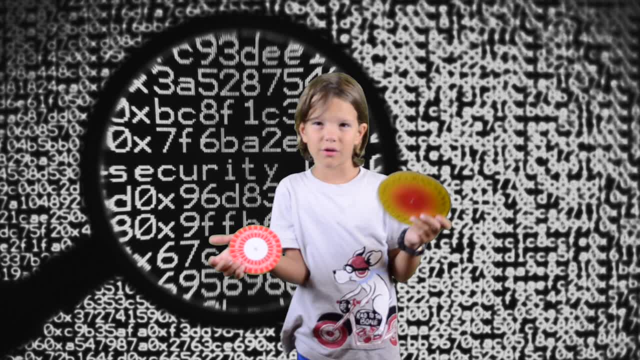 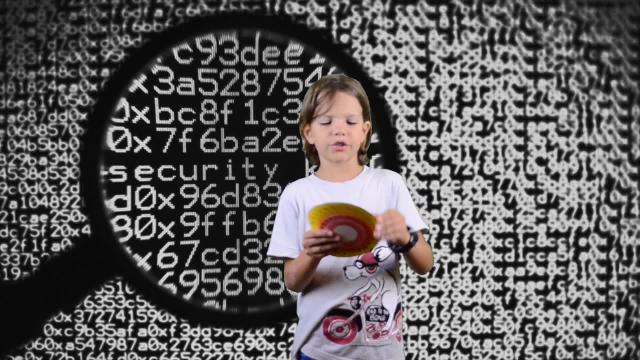 You can go. You can see some free print, Some free printable Printable two wheel. Two wheels with the setting up of a cryptography wheel. So when you print it out, all you basically need to do is First just cut it out. 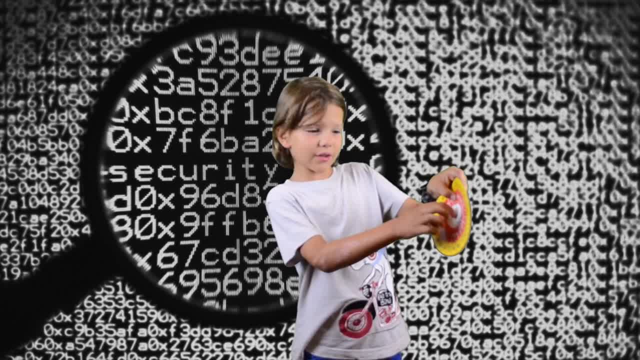 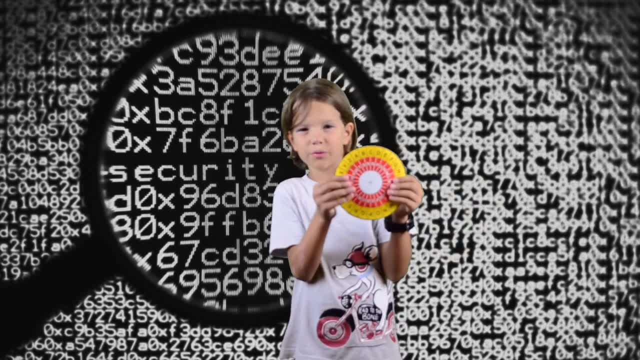 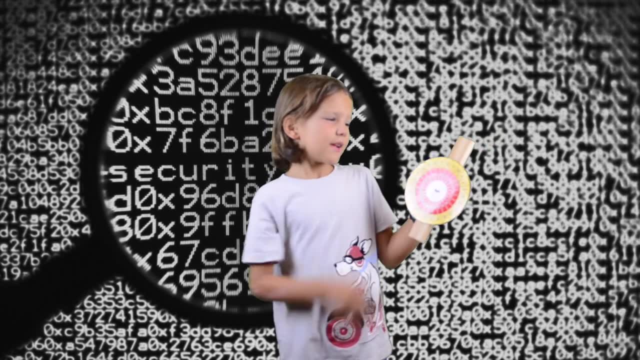 And then make, And then make two holes in the In the middle of, In the middle of both of the papers, And put them together. And first you just put them together and it will look like this, So to have an actual sniffer disc so you can turn around. 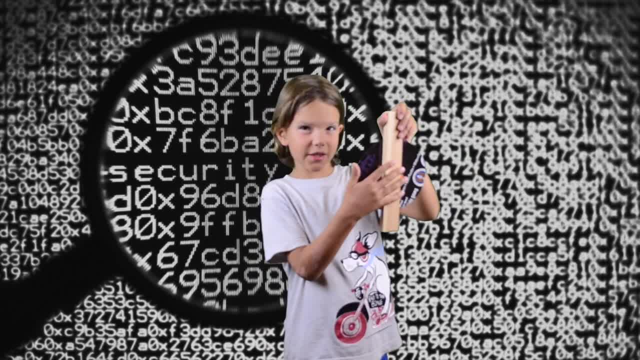 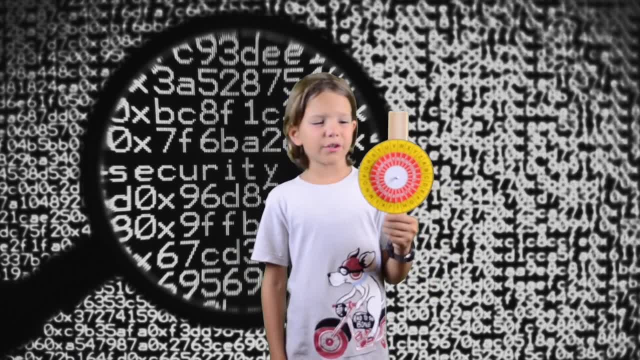 I just got a wooden, A wooden little stick, as you see on the back, And just screwed it with a nail And, of course, everyone that you're, That you're taking secret, That you're giving secret messages to, will need this. 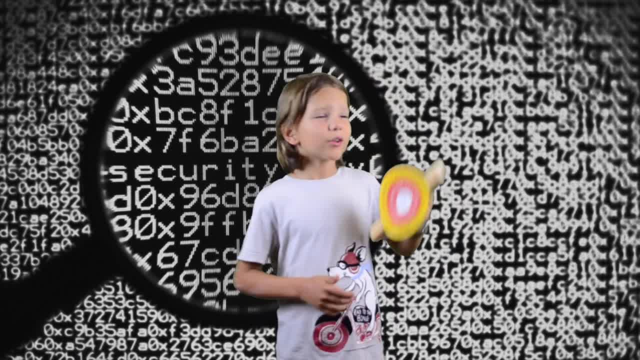 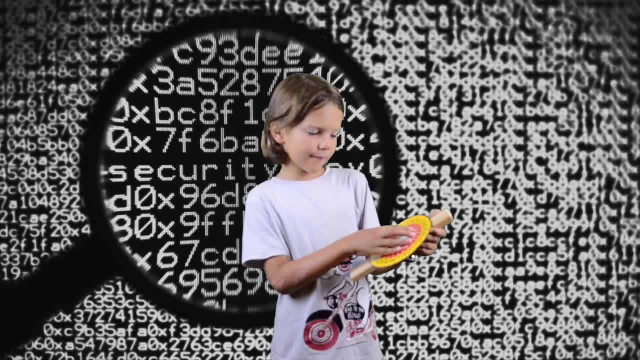 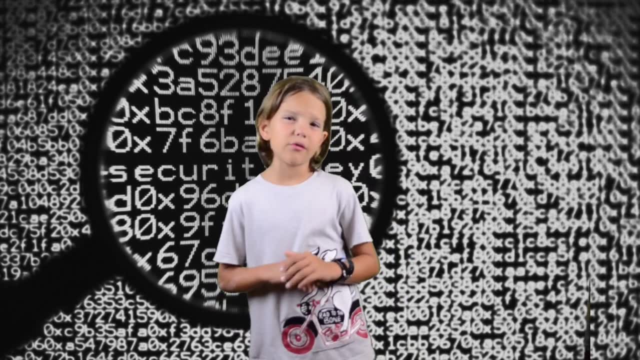 One thing you need to obviously do is tell your person Is tell the secret key. For example, let's just set mine to BL. Then the other person, you tell them the key and they can decrypt it. Now let me explain you how to. 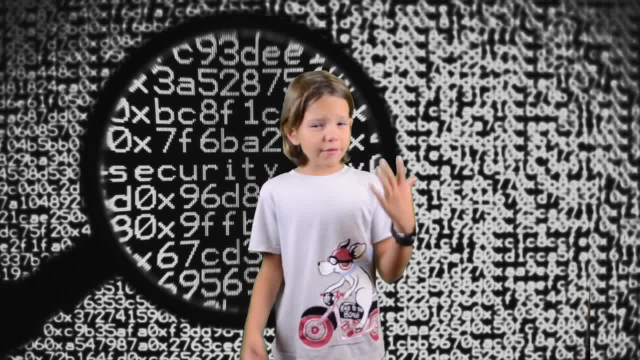 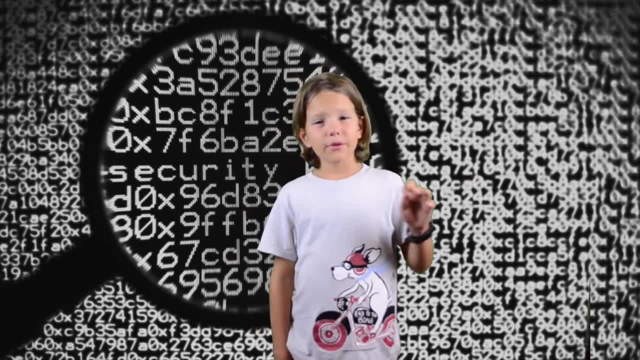 How to win the $25 Amazon gift card. In my video there was a secret hint word, Not Not a huge message, but just a word. So if you re-watch my video and watch it very carefully, Then Then you're gonna see some words. 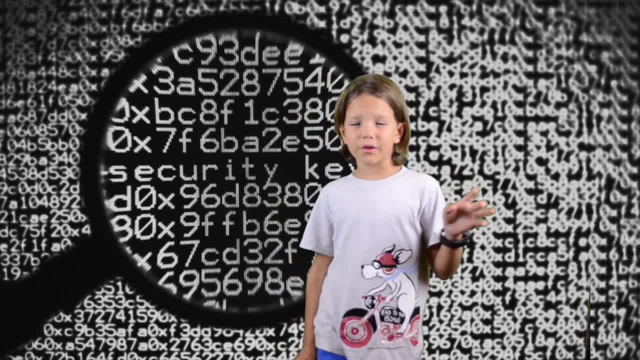 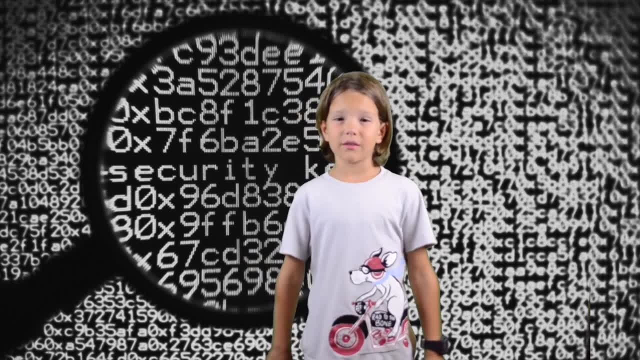 Or some letter clues, And when you, When you put them all together, You're gonna, You're gonna get, You're gonna get a word that you're probably really easily gonna Gonna find. And when you find the word, Go in my description and there's gonna be. 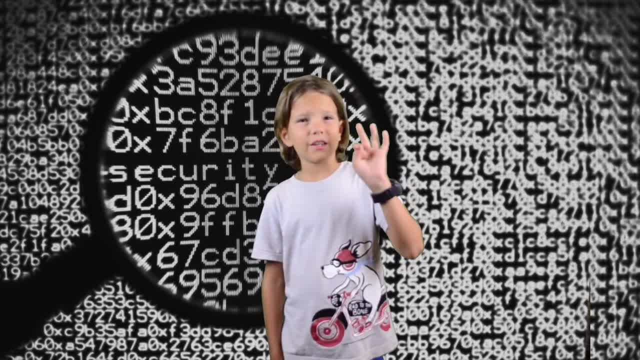 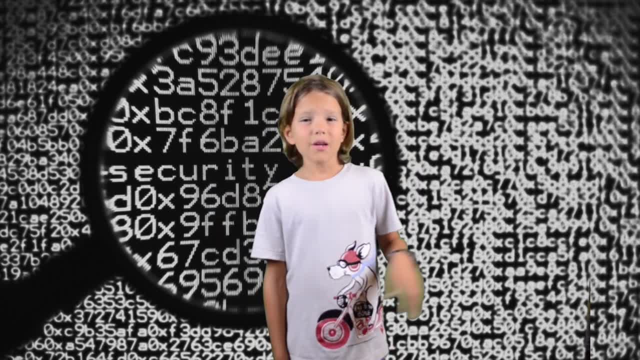 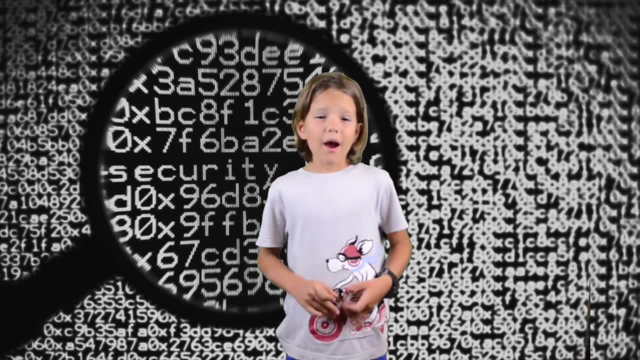 There's gonna be a link there, Click on it and the The title is gonna be submit- Submit- secret word. Click the link, Fill out the form And click the submit button. Don't forget to provide your email address, Because if you win, 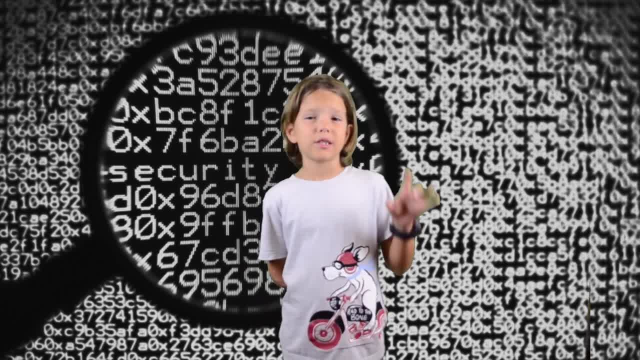 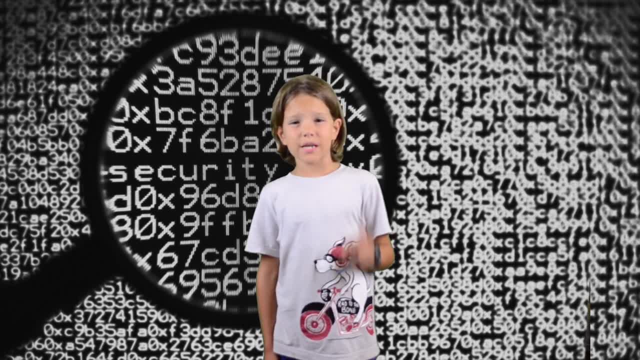 I'm gonna send, Because if you win, I'm gonna send it to your email. I'll give you. I'll give you three weeks for this task And the due date will be September 15th 2018.. If there is one, 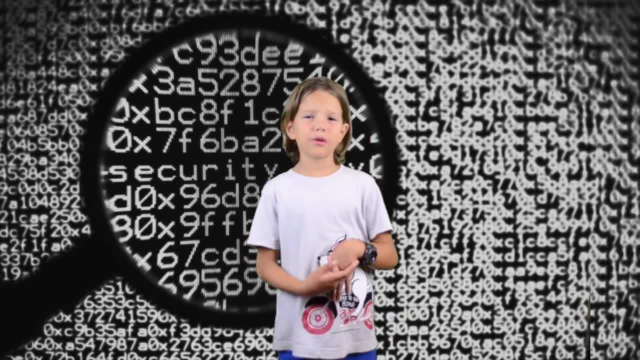 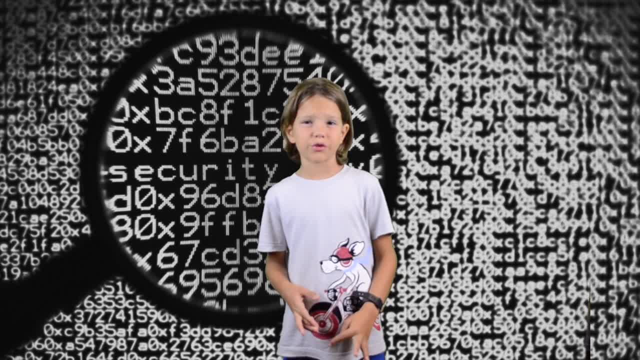 More than one person that got the word correct, Then we just do a random selection. But please don't put your answer in the comments. You can do it in the description, as I told you, Because in the comments You- I mean you- could just say: 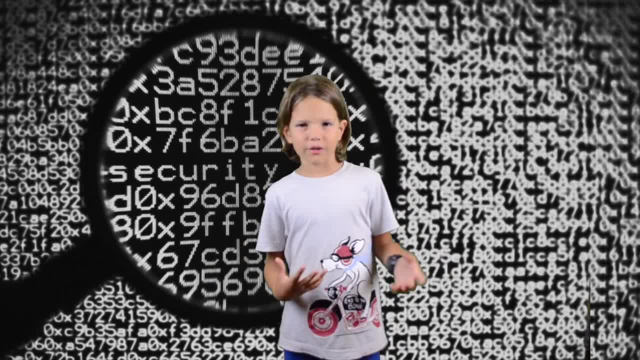 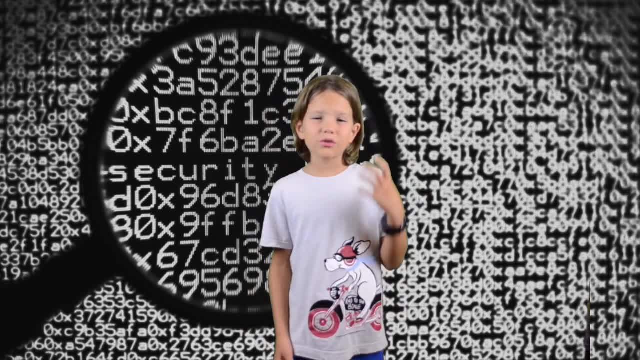 I. I found the word Uh Yay, So Don't say that you found it. Well, yeah, And you can say: I put it in the description, But please don't say that you found What the word is. 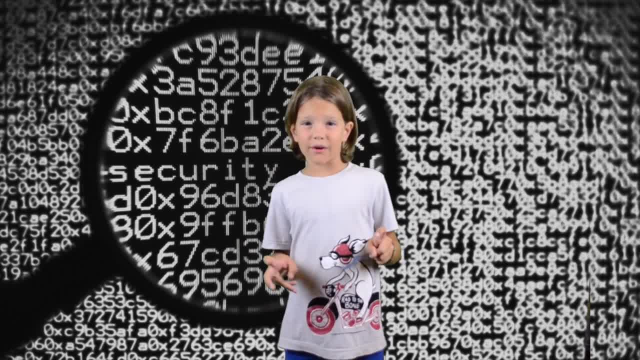 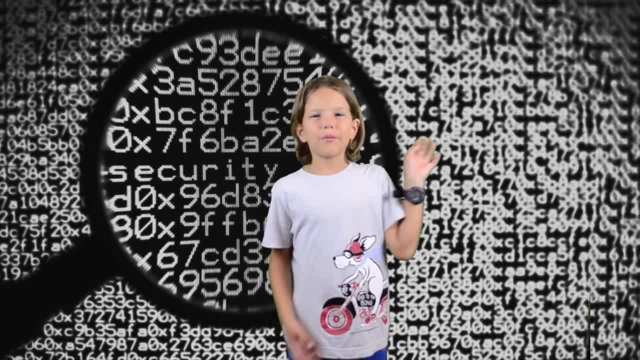 In the comments, because Everyone can scroll down in the video and see What the word would be. So good luck. Watch my channel about More photography, Technology, Robotics And much, much more. Bye.